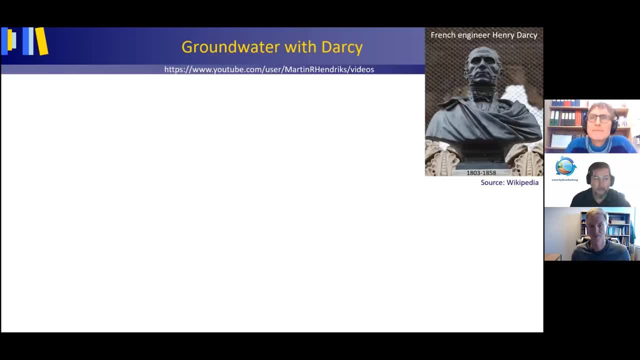 The question that came in had to do with mining. We saw, with Martin's example there, a river channel. Do you see any differences to those figures that were presented? when you're analyzing a mining pit, What if that was just a really, really deep hole, Would it look the same? Those 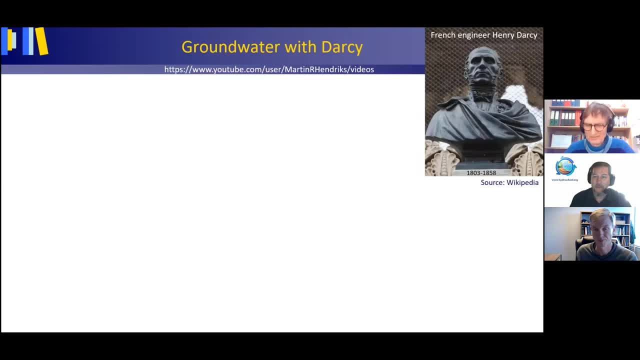 same principles apply whether you've got a river sucking the water out of the system or whether you've got a mining pit that's being pumped out. Any applications there from your background that you wanted to share with us? Yeah, if you have open pit mining, I guess it would depend if the 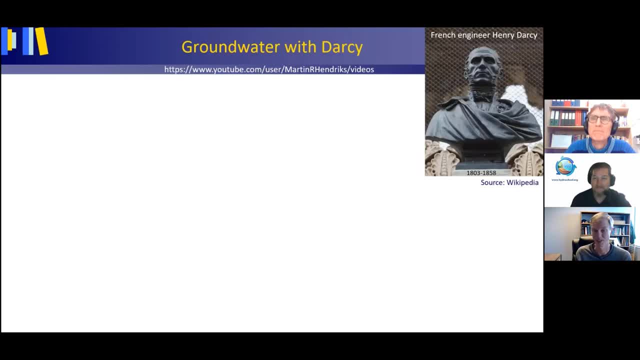 pit itself would become a terminal sink or not. And what I mean by terminal sink is whether water will flow back into the pit, or will it be a flow through pit, where it will just continue to flow through, like Martin showed in his example, and it would continue to go to the discharge point. 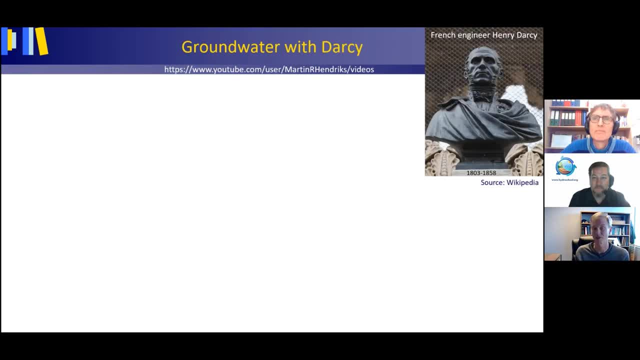 which is a river. You assess that typically through predictive numerical modeling and look and kind of calculate a new quasi-steady state once you stopped mining and look at the recovery periods. So yeah, it's very applicable- the first principles that Martin's talking about- to mining. 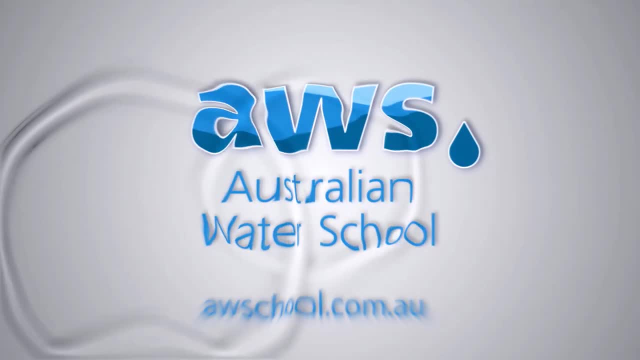 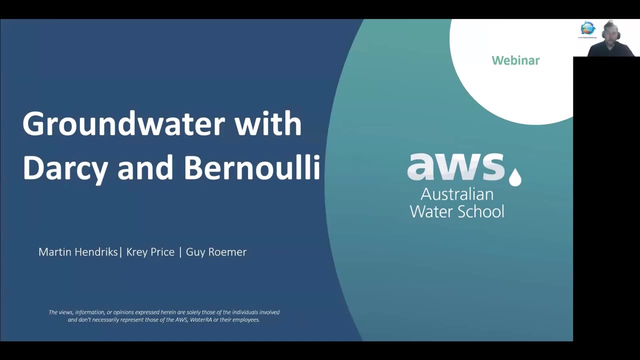 as well. Well, hello, I am Cray with the International Water Training Institute and, on behalf of the Australian Water School, welcome to the very first free webinar of our 2023 series. Today, we're going back to the basics with groundwater, whether it's new material for you or whether it's. 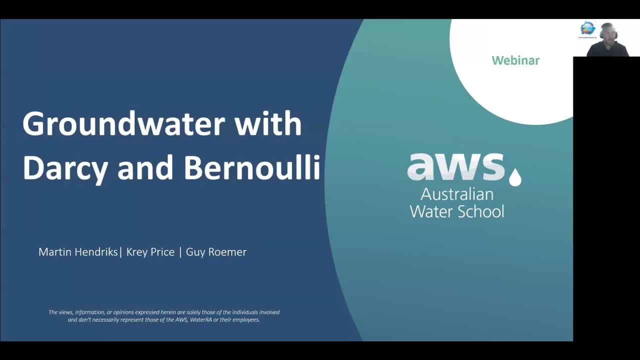 a refresher, whether you're a beginner or an experienced modeler. we're hoping that today's content can help fill any gaps that might have come into play since your last university course on the subject. So today we've got a global audience with us, So thank you for everyone. 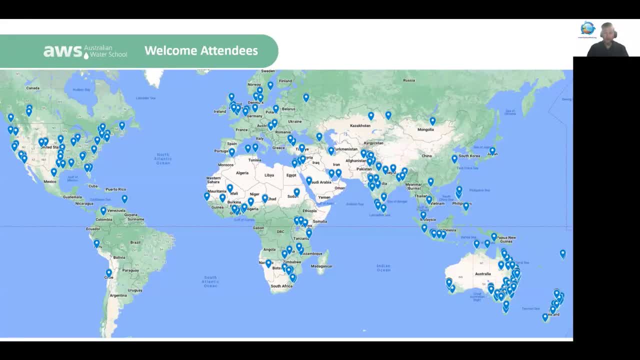 for your attendance, For those who are watching on YouTube later on- truly a global spread here, from all continents. If groundwater is an issue for you, we're hoping that the content that we give you today can help you wherever you are in the world, And thanks especially to those who 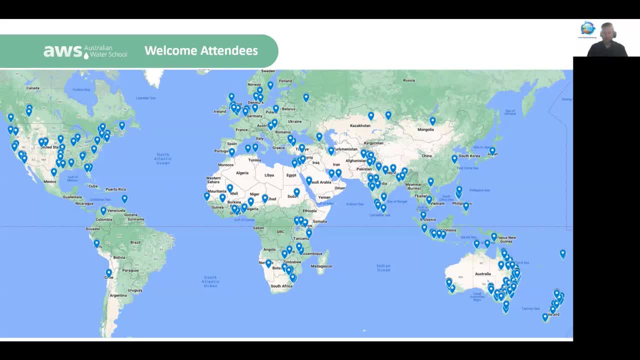 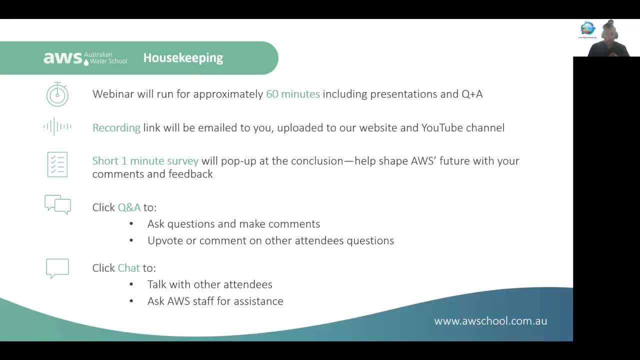 are joining us in the wee hours. on the chat line I can see some people who are joining us at two in the morning. Thanks for your participation in this and the efforts in sharing this time with us. So let's introduce our experts today: Martin Hendrix and Guy Rummer. Martin helped us out. 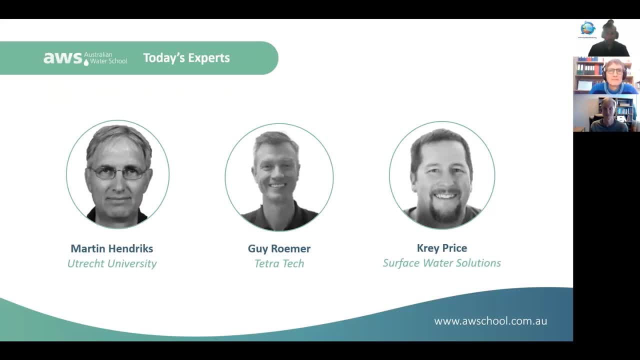 with a couple of courses in the past, So we're glad to have him back with us. And, Guy, this is his first appearance here on the Australian Water School's webinars, So to both of you, I guess, just if you could give us a brief introduction where you're coming to us from today and how. 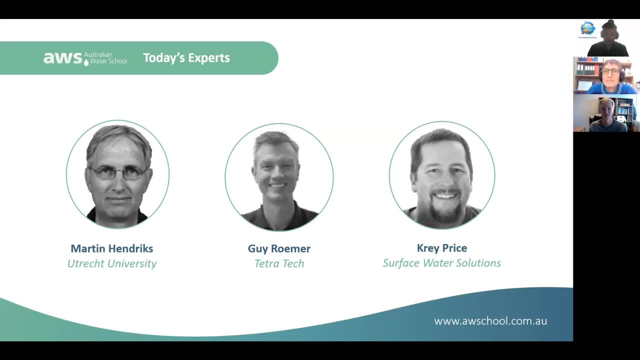 long you've been doing, how long you've been in the groundwater business, Martin, first to you and then over to Guy. I'm coming from Apkoude, a little village in between Amsterdam and Utrecht. Basically, I've been. 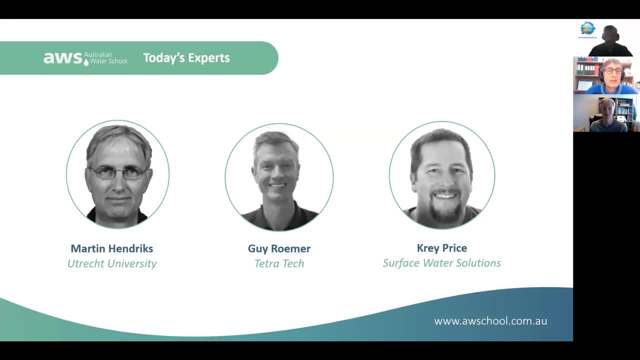 working at universities for more than 30 years. I'm retired now And I did a lot of lecturing in hydrology, mainly groundwater hydrology. Also, I was involved in landslide research- research linked to climate change- So I managed to put up an education system where I would warn the students for the 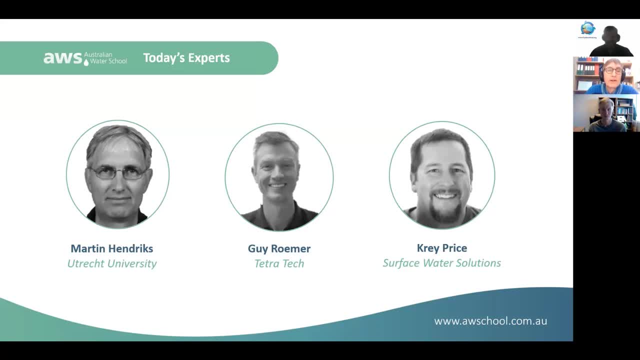 pitfalls of hydrology because there are many, especially at the beginning. So I'm very pleased that I can give this lecture and take away, maybe with the beginners, But it's a very wide audience. There may be people who are really I don't know. I don't think there's a way into groundwater modeling. I don't know, We'll see. 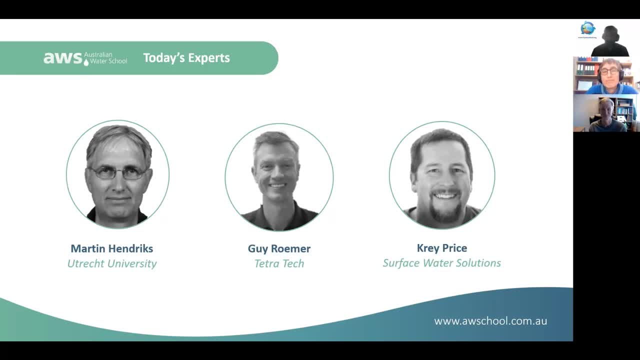 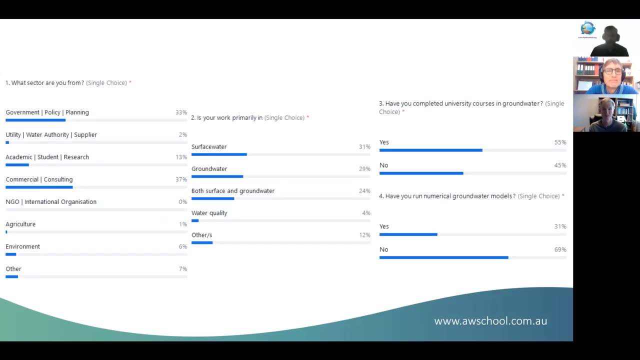 We'll have a little bit of a poll actually in the meantime, So that'll give us a good feel for what level everybody's coming to us from. So if you filled out that poll in the beginning, thank you, Maybe we'll have a look at those results while Guy's introducing himself. 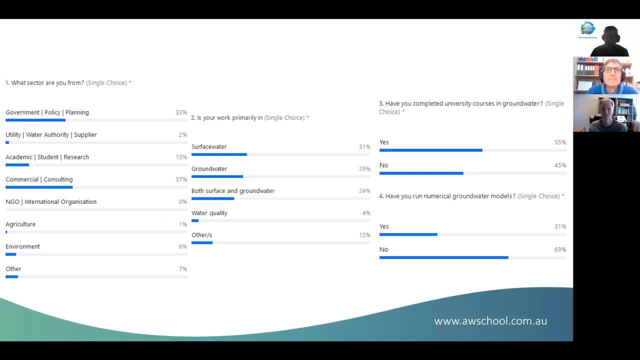 And, Guy, maybe just let us know, as you're looking through here, if you have any surprises. Yeah, sure, Yeah, it looks like We have 31% that have ran groundwater models before. So that's exciting for me because I'm a. 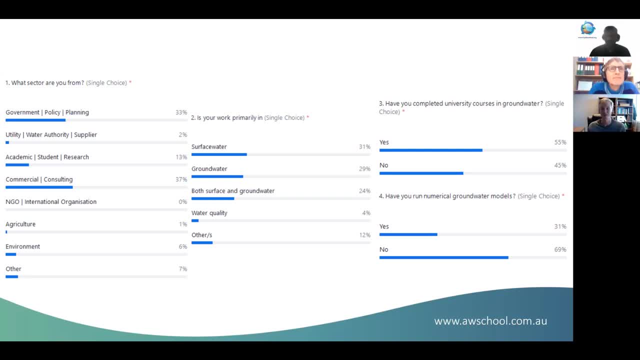 groundwater modeler. So yeah, So I work with Tetra Tech. It's an environment consultancy firm pretty global. It was even over in Australia, in Perth, for a year and a half with CRAE. But I've been doing groundwater modeling since my master's degree. I started off at Los Alamos. 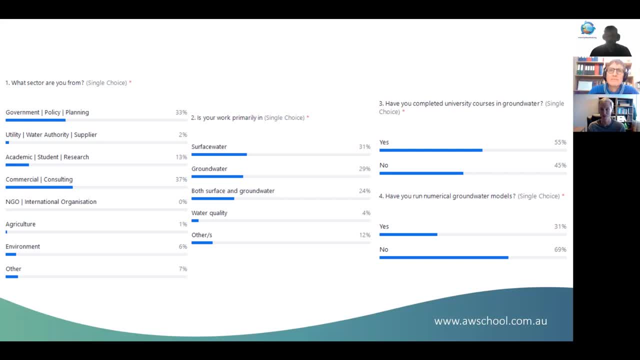 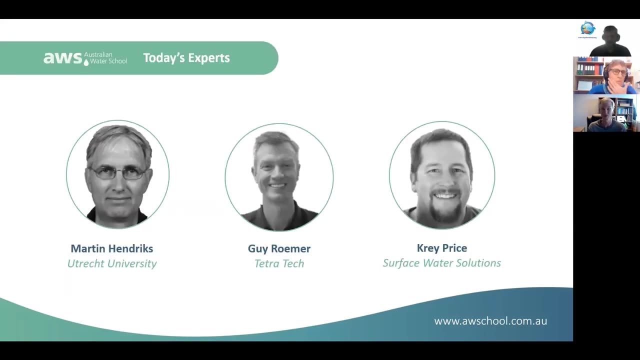 National Laboratory doing groundwater flow and solute transport modeling for Yucca Mountain, which was the proposed level waste, you know, nuclear repository in the states. and then i started with tetratech in 1999 and i've been doing groundwater modeling ever since, mainly for commercial uh industry. so for 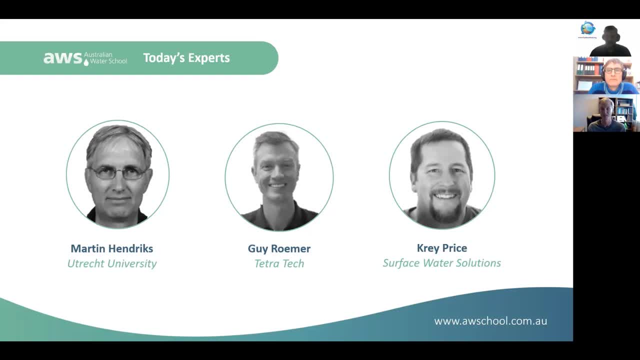 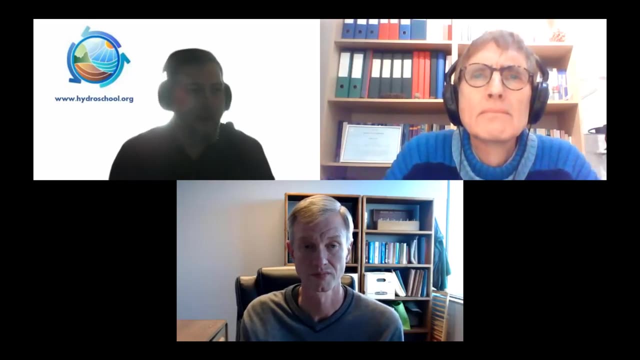 mines, oil and gas contaminated sites, you name it. i've probably touched it at some point in the last 25, 26 years. excellent, all right now, while martin's getting ready to share his screen. martin will be our main presenter today, but, um, i wanted to just mention that. um, you know, this year, uh, for our 2023. 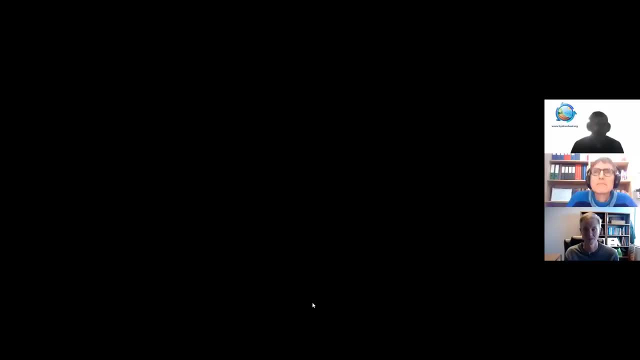 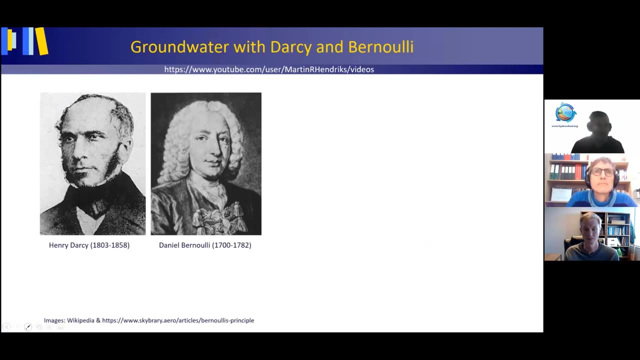 webinars. we're going to try to continue to build on some of our key disciplines with you know: groundwater, surface water, water quality. we're going to be bringing you a whole range of new topics- tidal energy, wind and wave forces, desalination- but we're also going to try to 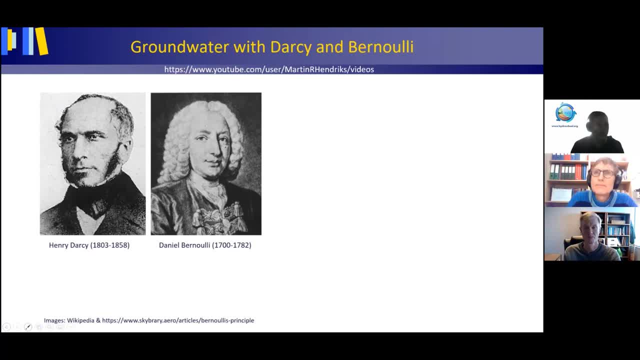 continue to expand some of our most popular previous topics with new webinars and courses that are going to cover qgis and heck razz, mod flow and some of the practical applications. um, we do try to balance a bit of the theory with the practical side of things. um, so you'll, i hope. 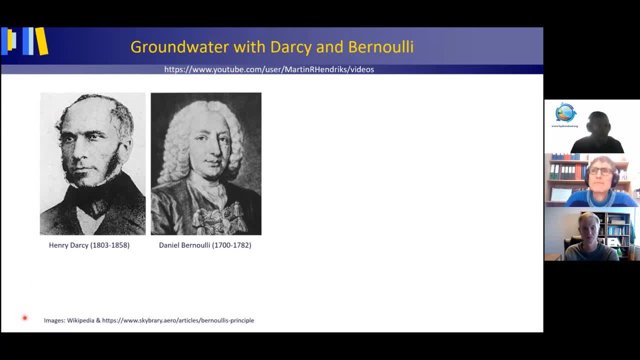 you get a feel for that today. so stay tuned for the registration links for some of those upcoming webinars. we'll provide those at the end today and, even though there are some gaps in this year's schedule, they're filling up quickly but we still have some opportunities to incorporate other 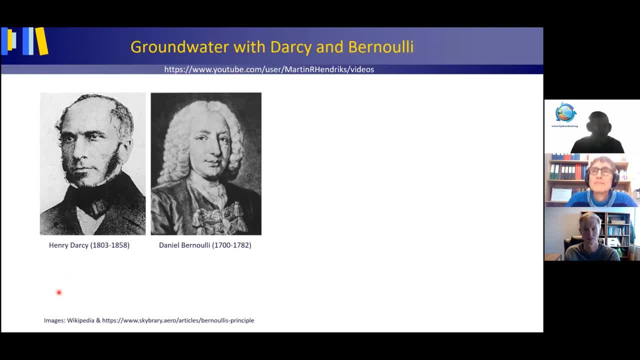 topics that you may want to hear about. so do not go, don't exit this webinar without giving us your feedback and let us know what you want to hear about. so on to today's topic. um, we are really excited to be introducing a new course called groundwater essentials. last year, with, with 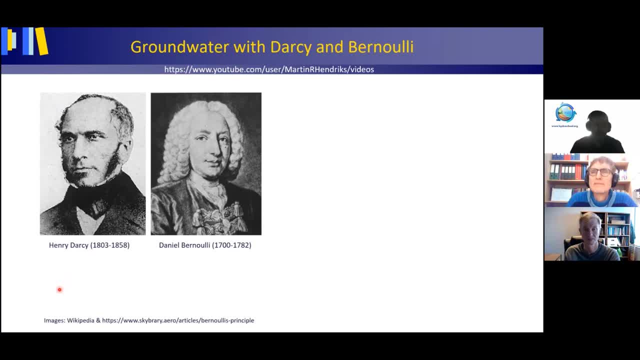 martin's help as well, we developed a course covering the essential principles of surface water hydrology and hydraulics. that's now available for on-demand registration, and we're going to continue that series with a groundwater essentials course that starts next month, and so, as an introduction to that course, today this is a free webinar that actually launches that course. 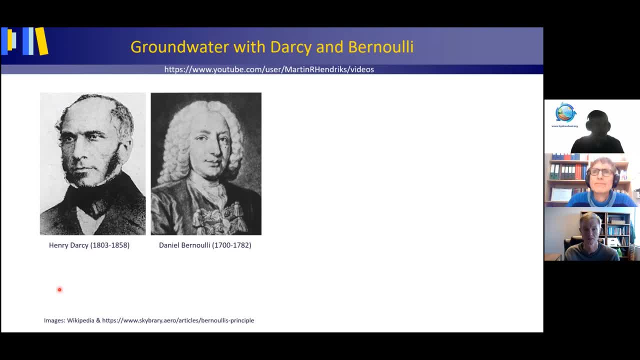 and we're going to meet martin as one of the key instructors of that course and we'll kick that off- this free webinar: some of the most fundamental principles involved in groundwater hydrology. So with that, Dr Hendricks is joining us in the late hours in the Netherlands. 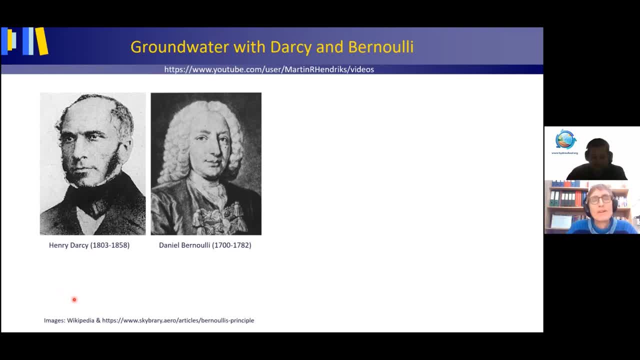 So with that I'll turn my camera off Over to you, Dr Hendricks. Well, thank you, Craig And everybody. welcome to this lecture on groundwater with Darcy and Bernoulli. Darcy lived in the 19th century and Bernoulli in the 18th century. 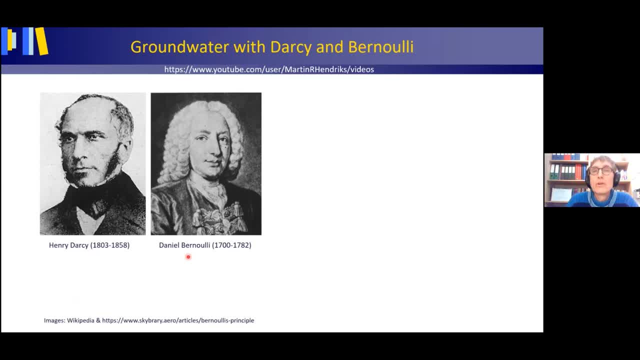 And understanding the equations or laws that they derived is fundamental to understanding groundwater hydrology. Well, first of all, groundwater is important as effluent seepage, seepage, leaving a groundwater body that feeds streams, rivers, wetlands and lakes. 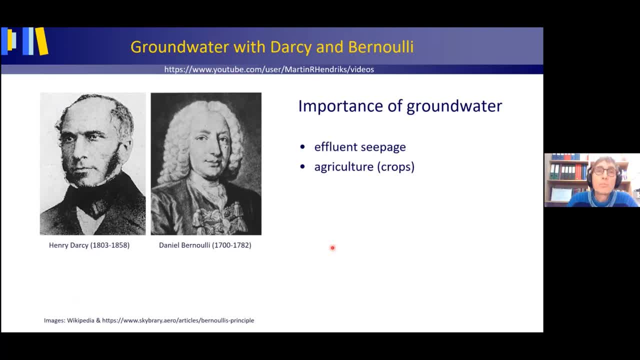 It's important for agriculture the growth of crops as an often clean source for drinking water and for many industrial activities, and for the sustainment of biodiversity in groundwater-dependent ecosystems. Groundwater is a valuable resource that needs to be protected from pollution and over-exploitation. 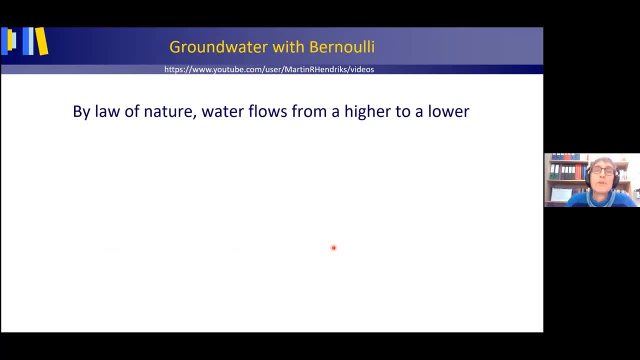 Let's start off with a little. Let's start off with a little quiz. a multiple choice question: By law of nature, water flows from a higher to a lower A elevation. Is that the right answer? or is the right answer? By law of nature, water flows from a higher to a lower B energy. 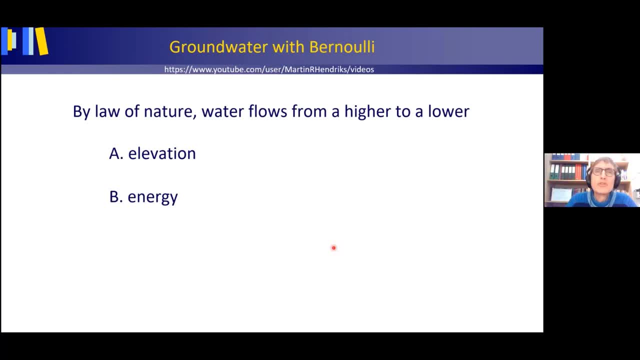 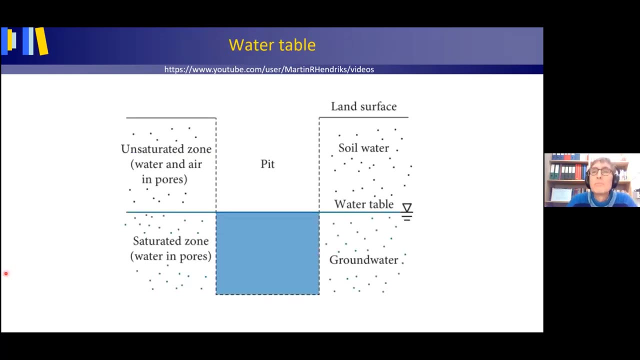 Or does water, by law of nature, flow from a higher to a lower water pressure? or are D all of the above options true? Think about this. To start off, we first need to explain the positioning of the water table in easy terms. If you were able to dig a large pit, the level to which the water from the ground rises in that pit. 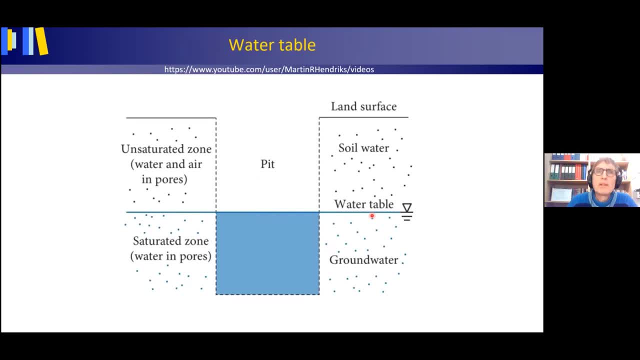 is called the water table. The water table is in between the, The unsaturated zone, with soil, water, water and air in the pores, and the saturated zone, or groundwater water in the pores, fully saturated water. A water table that can establish itself freely is, by definition, the level at which the pore water pressure in the ground equals the air pressure of the overlying air. 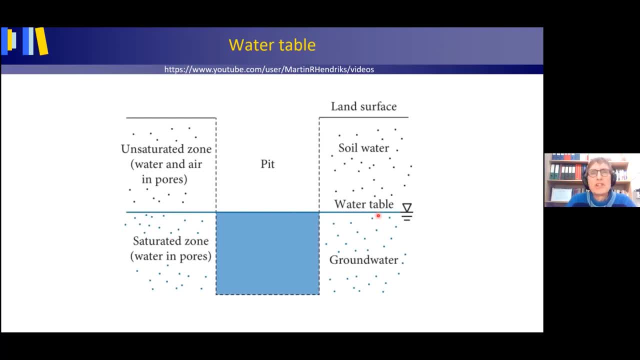 On average, this air pressure is the standard atmospheric pressure of one atmosphere, which is 1,013.25 hectopascal. Instead of using this a little bit awkward standard value as the average water pressure at a free air-water interface such as this water table, 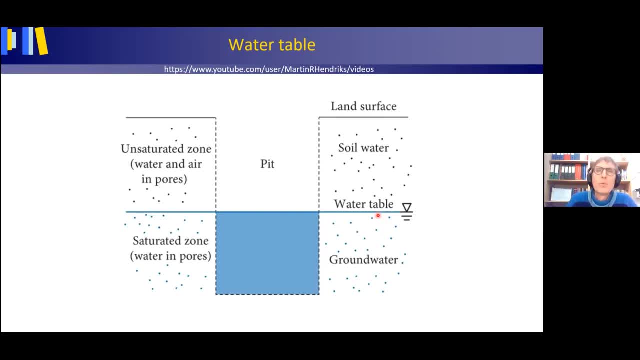 it is a common practice to define the water pressure at a free air water. Thus, the water pressure has a value that should be interpreted with the existing air pressure at the air-water interface as a reference, And the zero water pressure means that the water pressure equals the existing air pressure at the air-water interface, as I said before. 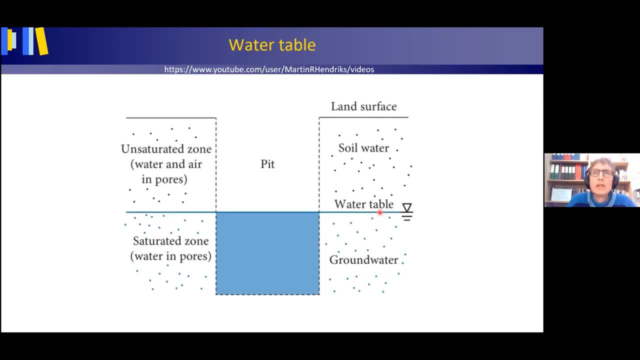 This is what we commonly do in hydrology. We simply denote the water table As having a relative water pressure zero, or, in short, as having a water pressure zero. When we move down into the groundwater, we have positive water pressures, And when we move upwards from the water table, we have negative water pressures. 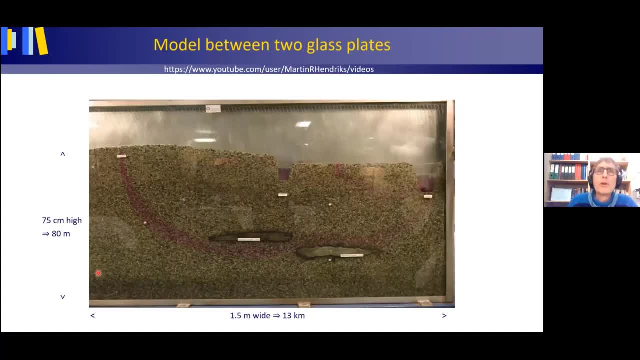 This photo shows the model shows a model between two glass plates. The glass plates are five centimeter apart And the space between the glass plates is filled with gravel and sand. gravel and sand. In reality, this makes for sand and clay layers. 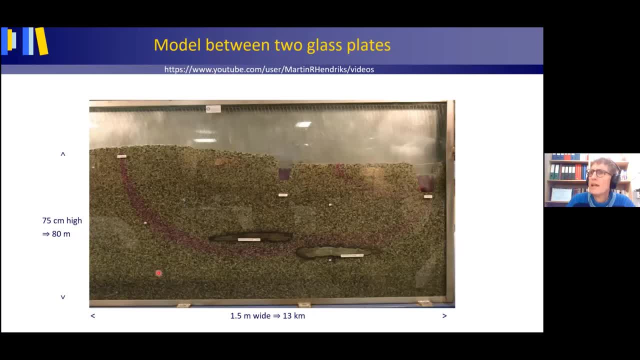 The model is 75 centimeter high and, at the bottom, one and a half meter wide. The model is a replica of the subsurface, being 80 meter high and 30 meters high, And it is 18 kilometer wide. To the left we have a higher part of the landscape. 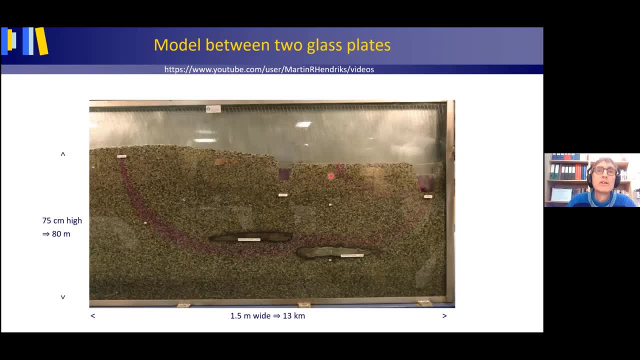 And to the right we have a lower flat part of the landscape. It rains, as you can see at the top, and water moves out of the model in a small stream in the middle and river to the right. From the back of the panel a coloring dye is injected into the system. 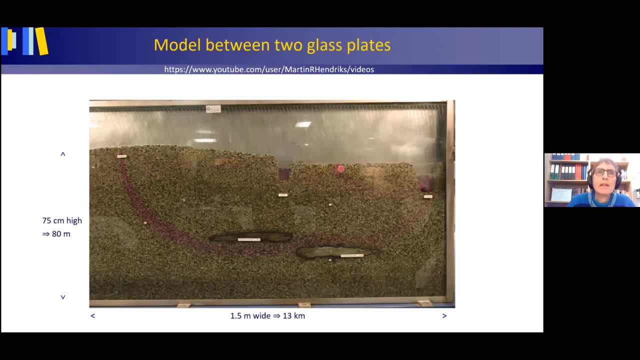 from the back of the panel, a coloring dye is injected into the system at 2 times. from the back of the panel, a coloring dye is injected into the system at 2 times locations. This enables us to follow the groundwater flow pathways. 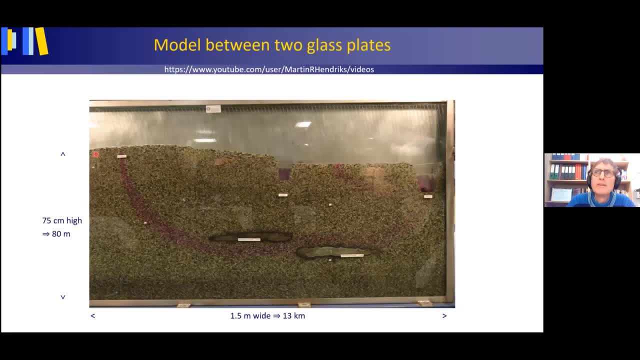 The water table is approximately as I'm indicating now, And the water table of course coincides with the surface water level at the stream and at the river. We see that groundwater from the left flows in this manner through these two clay lenses and then into this river. 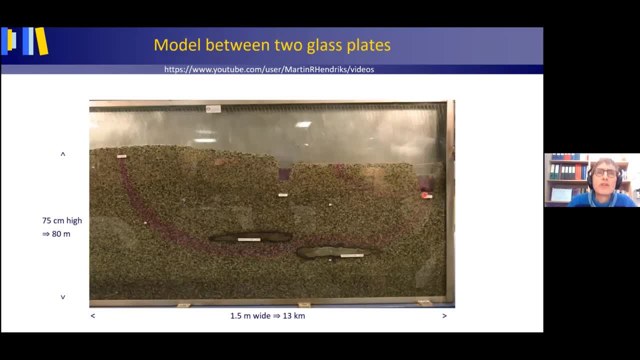 We call this a regional flow line. At the top of the subsurface we see the movement of the groundwater along a local flow line. Let's take a better look. What do we actually observe? First, we see that in this setup of phreatic or unconfined groundwater, 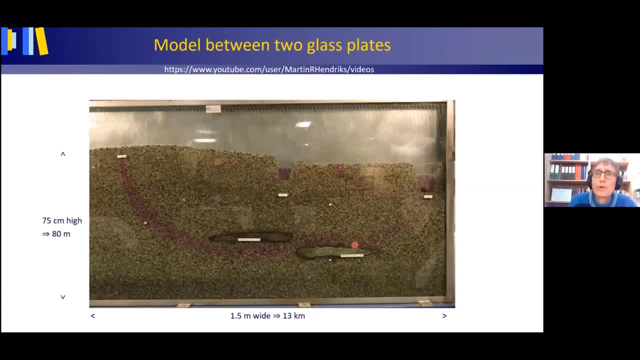 as it's called. groundwater flows along curved pathways, be it that curvature in this model is exaggerated, as the vertical height is exaggerated in comparison to the horizontal distance. Secondly, we see at the discharging end of the regional flow line that water flows from a lower to a higher elevation. 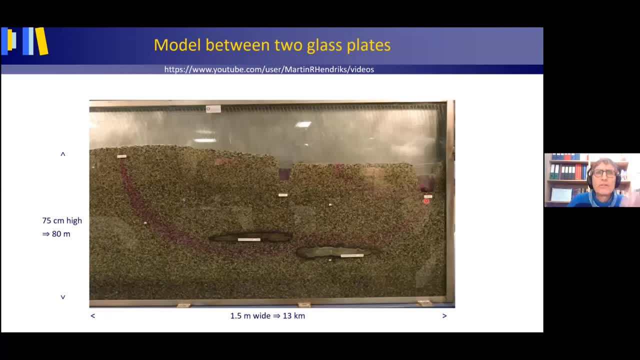 So there is no problem in that rivers may be fed from the groundwater below, Because the column of groundwater is larger. when we are deeper down in the subsurface, the water pressure is larger deeper down. Thus we observe at this discharging end: that the groundwater flows from a higher to a lower water pressure. If we look at the recharging end, we see the opposite: Groundwater flows downwards from a lower, thus to a higher water pressure, So there's no problem in that too, as well as from a higher to a lower elevation. 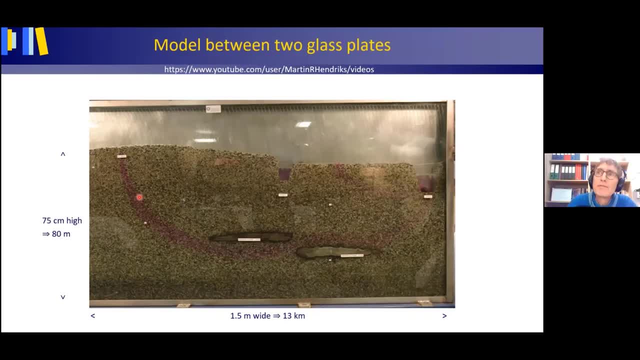 In conclusion, groundwater can flow from a higher to a lower elevation, From a lower to a higher water pressure, But also from a lower to a higher elevation, From a higher to a lower water pressure. So we now know for sure that two of the options in the multiple choice question. 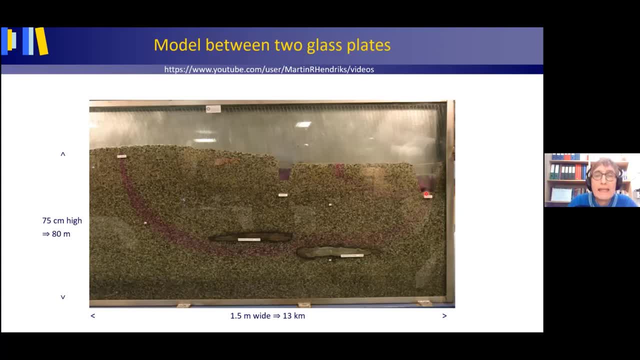 by law of nature, water flows from a higher to a lower elevation and C, from a higher to a lower water pressure are not true. This also rules out option D. All of the given options are true. Thus, by law of nature, water flows from a higher to a lower energy. 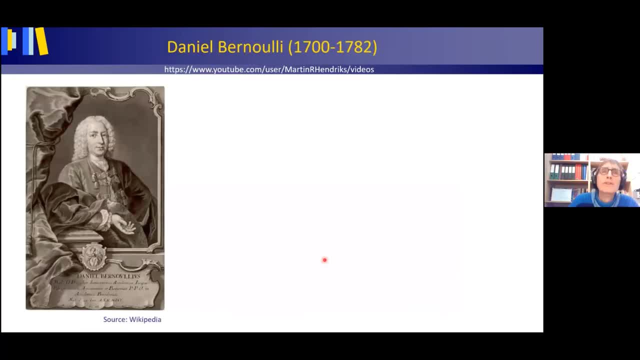 Answer B: Daniel Bernoulli is a Swiss mathematician and physicist, born, by the way, in the Dutch city of Groningen. And to better understand the physics behind groundwater flow, let's now continue with Bernoulli's principle. Let's first take the example of water flowing through a garden hose. 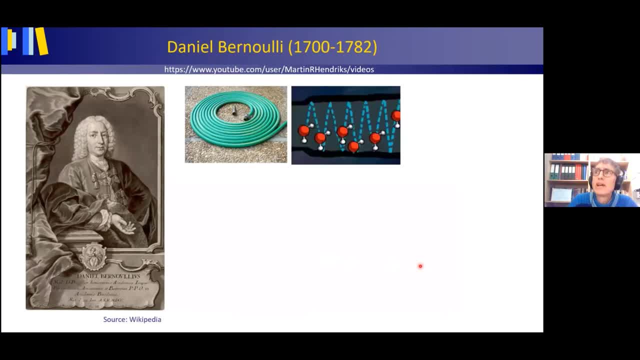 Water molecules collide with the inside of the garden hose, building up static pressure. If the water moves slowly, we have many collisions and a higher pressure. If the water moves fast, we have fewer collisions and a lower pressure. In fluid dynamics. Bernoulli's principle states that an increase in the speed of a fluid 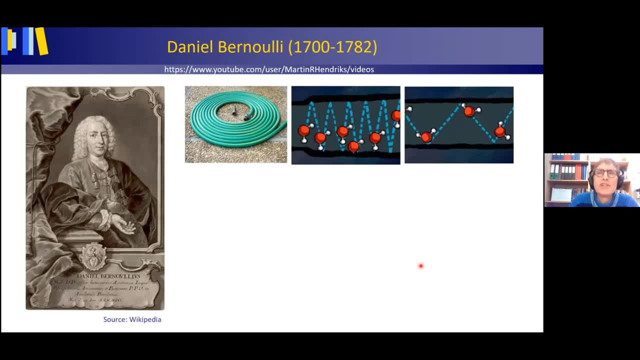 here, water occurs simultaneously with a decrease in static pressure or a decrease in the fluid's potential energy. Another well-known example is provided by air rushing around the wings of an airplane that is speeding up on the runway. The wing's upper surfaces are curved. causing the air rushing over the top of the wings to speed up, which decreases the air pressure above the wings. The pressure on the top of the wings, then, is less than the pressure on the bottom of the wings, and the end effect being that the wings are lifted. 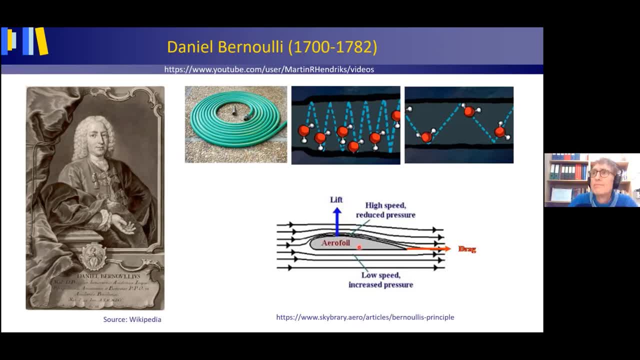 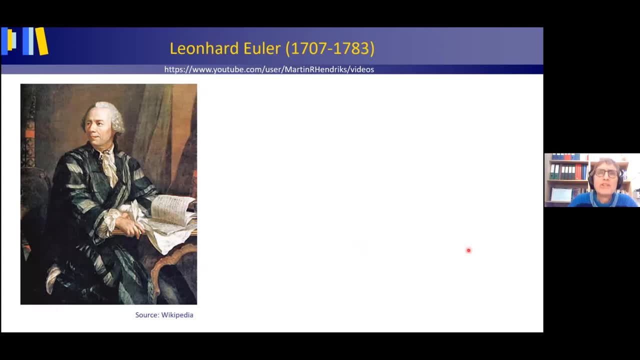 and the plane takes off into the sky. Although Bernoulli deduced that pressure decreases when the flow speed increases, it was Leonhard Euler, also a Swiss mathematician and physicist, who derived Bernoulli's equation, or law as we know it. 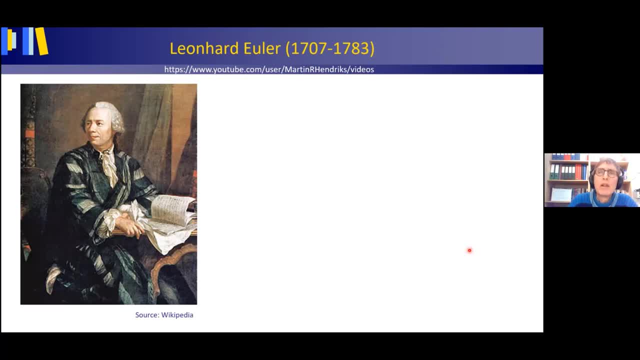 A water particle moving along a streamline possesses three interchangeable types of mechanical energy, all in joule: Kinetic energy, potential energy and pressure energy. m is the mass of the water in kilogram small v is the velocity in meter per second. 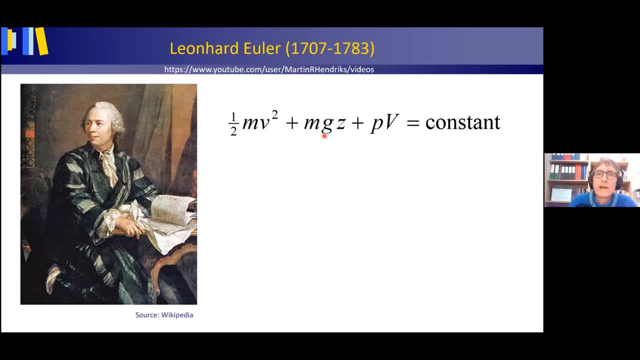 g is the acceleration due to gravity in meter per second. squared z is the elevation in meter and p is the pressure in joule per cubic meter or newton per square meter. Large v is the volume of the water in cubic meter If there is no loss of mechanical energy due to friction. 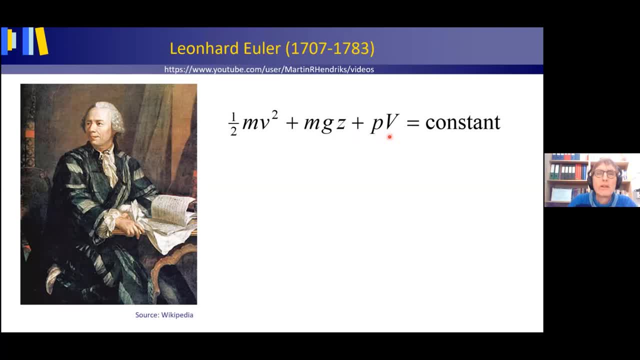 and if we take water as incompressible, then Bernoulli's law for steady flow states that the sum of these three interchangeable types of mechanical energy is constant, A notion also known as conservation of energy, and Bernoulli's law is also sometimes referred to. 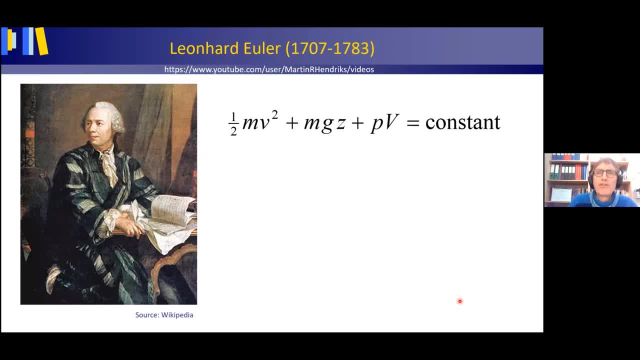 as the energy equation. As flow velocities in groundwater are observed to be very slow- I'll come back to this later- the first term, the kinetic energy, may be neglected and thus for groundwater, mgz plus pv is constant. By dividing all terms to the left and the right, 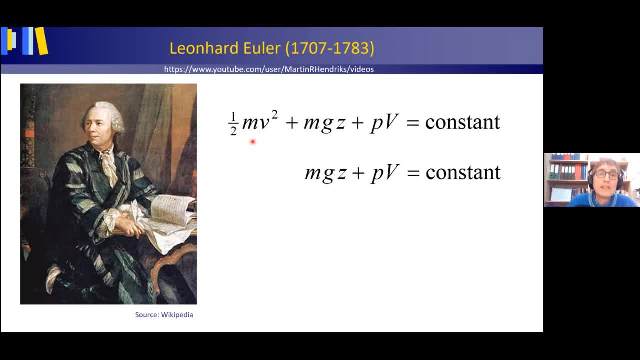 of the equal sign. by the volume, large V, we obtain an expression per unit volume of the water. Mass m divided by large V becomes density, rho. so rho gz plus p is constant, Because fresh water has a constant density of 1000 kg per cubic meter. 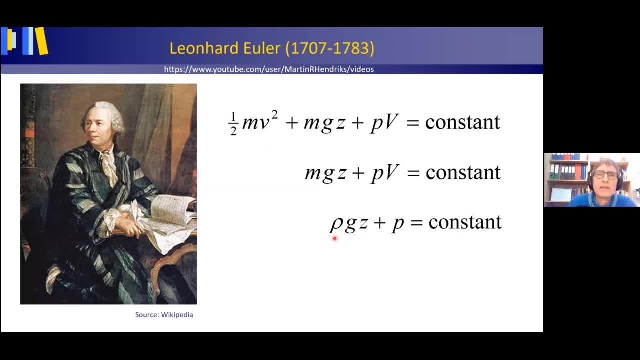 we can also divide by the density, and because g- the acceleration due to gravity at a certain location- is also constant, we can also divide by g. This delivers the following equation: z plus p divided by rho- g is constant- in which all mechanical energy terms are presented. 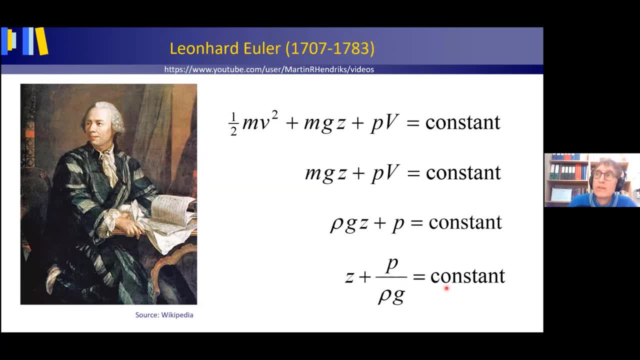 in the length unit of meter, Z is called the elevation head. p divided by rho, g is the pressure head and the constant length unit to the right of the equal sign is the total energy. with the length unit, the hydraulic head, We can quite easily measure the hydraulic head. 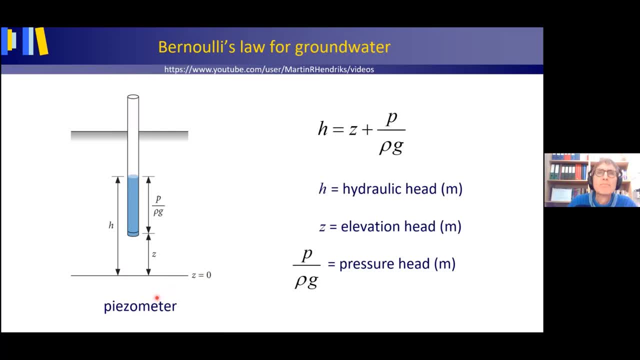 by using a so-called piezometer, which is a tube often made of PVC with a diameter of 20 to 50 mm and with a short screen of 10 to 30 cm length at the bottom, placed under the water table, through which groundwater enters the tube. 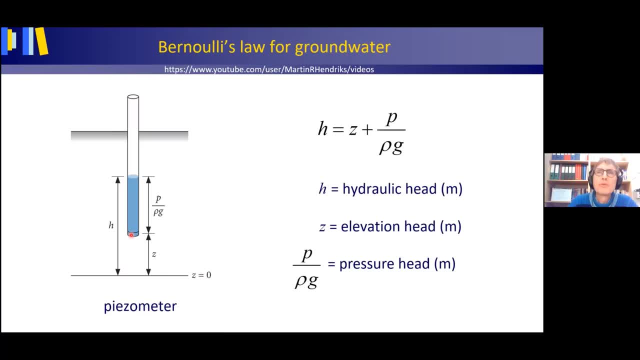 Groundwater can only flow into the piezometer through the screen at the bottom of the tube. The hydraulic head is thus measured at the location of the piezometer screen. Z is the altitude of the screen above the reference level in meter p, divided by rho. g is the water pressure. 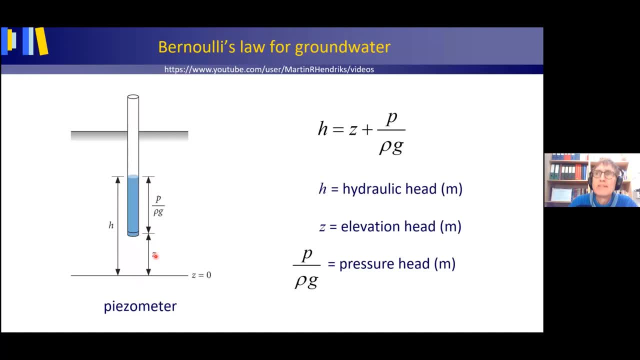 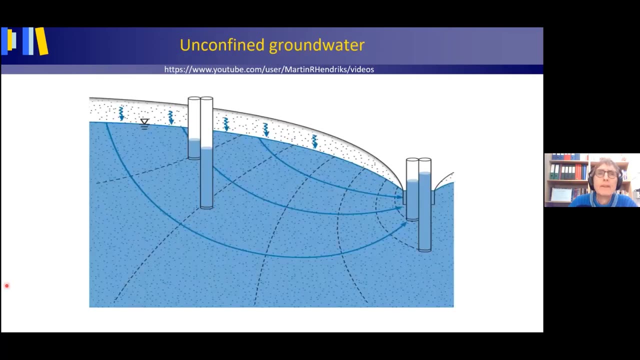 above the screen in meter and by adding z and p divided by rho g together, we obtain the hydraulic head in meter, the total energy as a length unit at the position of the screen. In this figure we see a phreatic or unconfined. 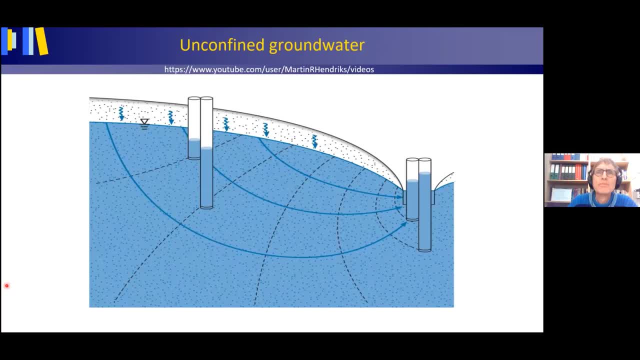 local groundwater flow system in cross-section. Here we have the surface of the land, the water table and a river or canal, and two pairs of piezometers at these two locations, with their screens at different depths. If we take the bottom of this picture, 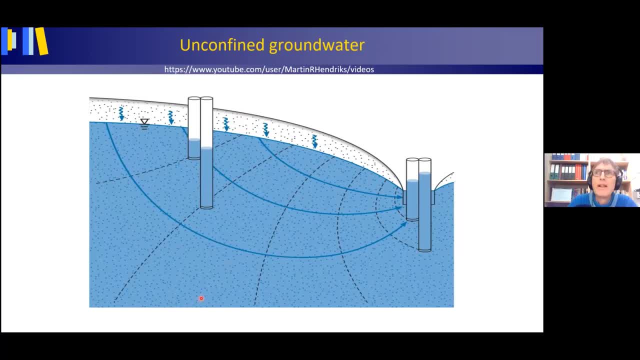 as our reference level. the hydraulic head measured at this piezometer screen is simply this height which I'm indicating with the pointer, And the hydraulic head at this piezometer screen is simply this height. So we have a higher hydraulic head here than here. 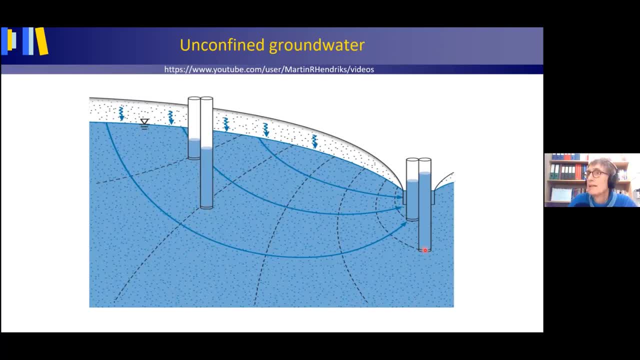 but we also have a higher hydraulic head here than here, So water is flowing downwards here and upwards here. Of course, with this right pair of piezometers you must take care that there is no leakage from the water in the river or canal. 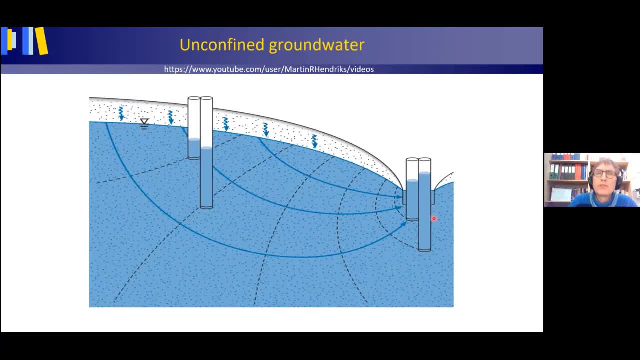 alongside the tubes. Important to mention is that for measuring a hydraulic head at the location of a piezometer screen, we must use a piezometer with a short screen, whilst for measuring the position of a free water table in a tube to mimic the level to which 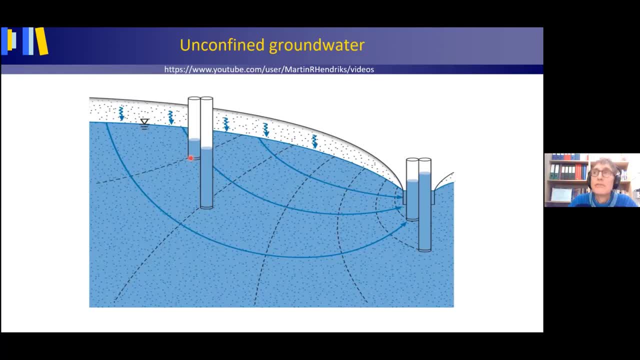 groundwater would rise in a large open pit. remember the earlier slide. the tube should be used that is perforated, thus acting as a screen all the way from bottom to top. If we were to install more piezometers, we could establish these streamlines. 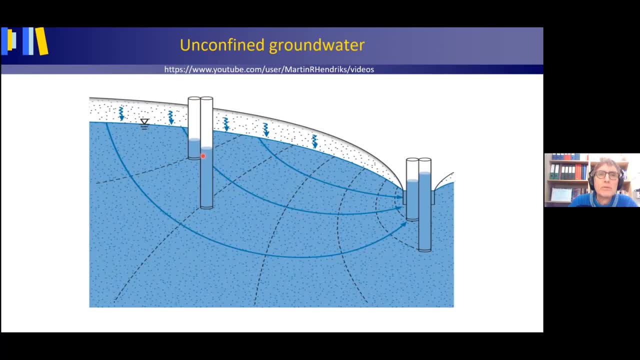 of the groundwater- Here it's recharging and here it's discharging into the river or canal- as well as the broken lines, which are lines of equal total energy or hydraulic head. These so-called equipotential lines are perpendicular to the flowlines. 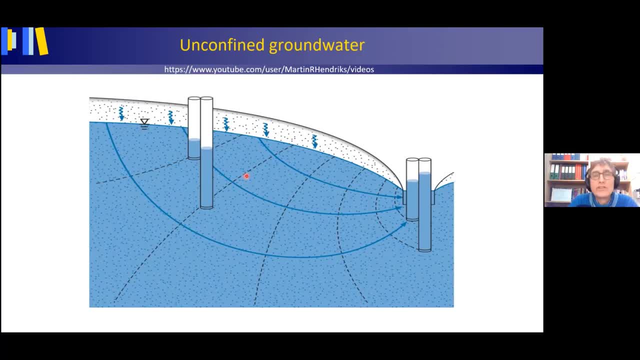 for steady groundwater flow, Which is defined as groundwater flow, for which the flow velocity components at any location do not change with time. So this is a higher hydraulic head, this is a lower hydraulic head, and this is an even lower hydraulic head, etc. 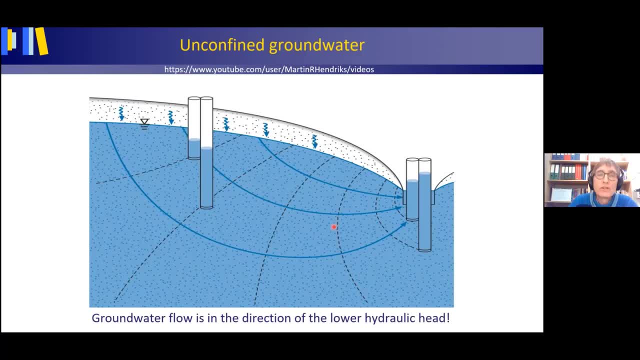 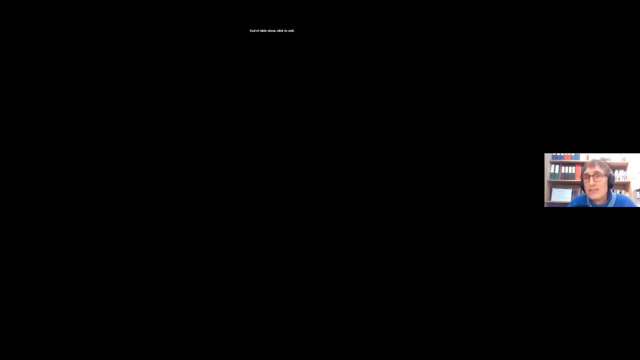 Again, the water always flows in the direction of the lower total energy, the lower hydraulic head, And this is the end of part one, So I'll turn back to Craig. Sure, yes, We'll have a follow-up to that. That was again. 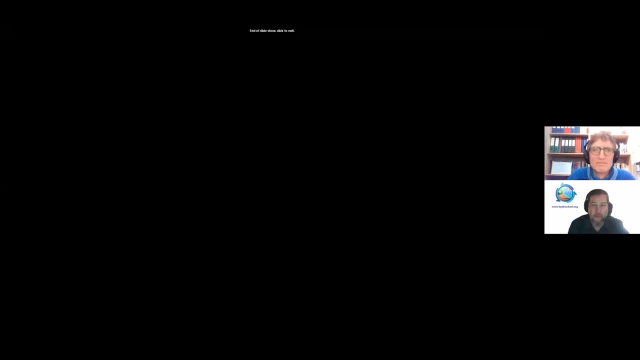 going back to the basics. We want to make sure that when we start a course like our Groundwater Essentials course, that everybody's got the same information going forward. And this is where it all begins with groundwater. Guy, if you wouldn't mind turning on your camera as well. 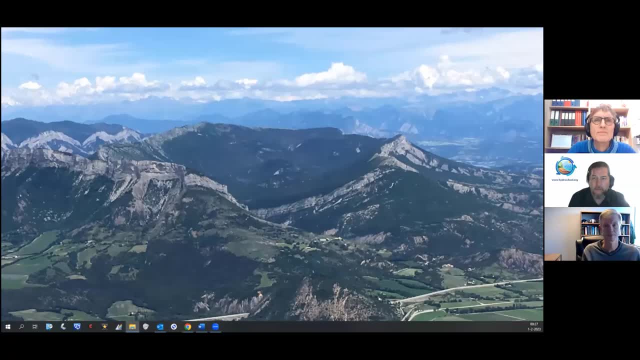 just maybe to highlight that question that you've answered in the background Now. I come from a family from more of a surface water background And, Guy, you've been in the groundwater side of things for a long time And a lot of people talk about. 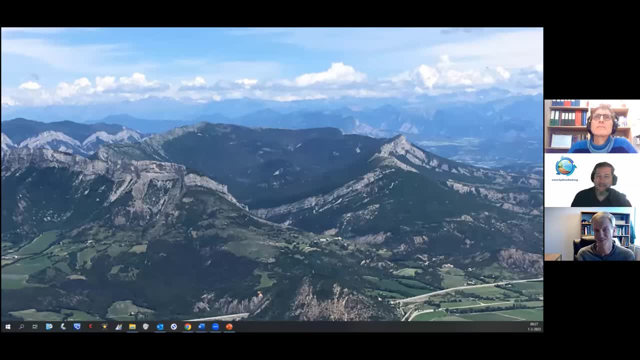 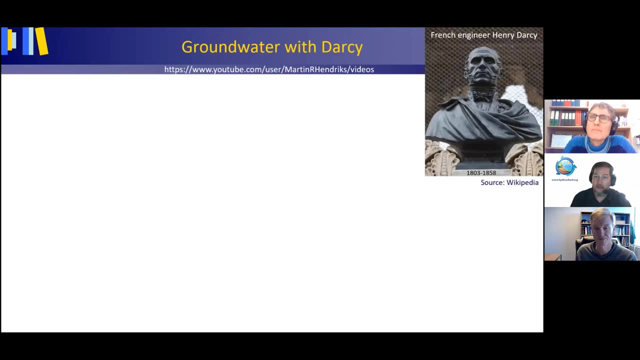 groundwater-surface water interaction And on the modeling side of things, that's a bit tough to do. The question that came in had to do with mining. We saw with Martin's example there, a river channel. Do you see any differences to those figures that were presented? 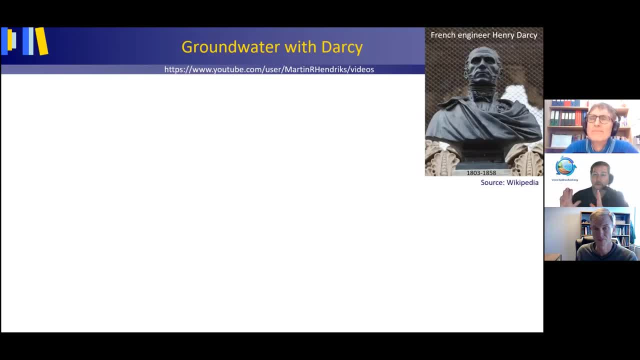 when you're analyzing a mining pit. What if that was just a really, really deep hole? Would it look the same? Do those same principles apply whether you've got a river sucking the water out of the system or what, Whether you've got a mining pit? 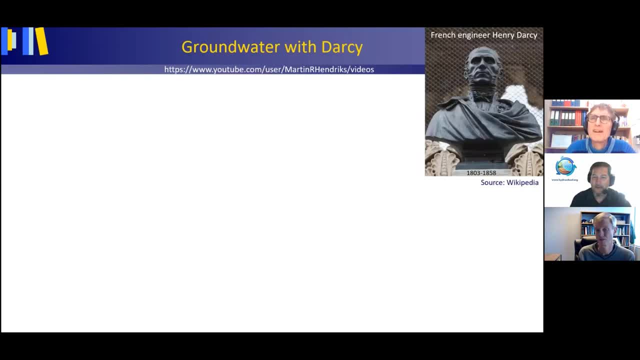 that's being pumped out, Any applications there from your background that you wanted to share with us? Yeah, If you have open pit mining, I guess it would depend if the pit itself would become a terminal sink or not, And what I mean by terminal sink. 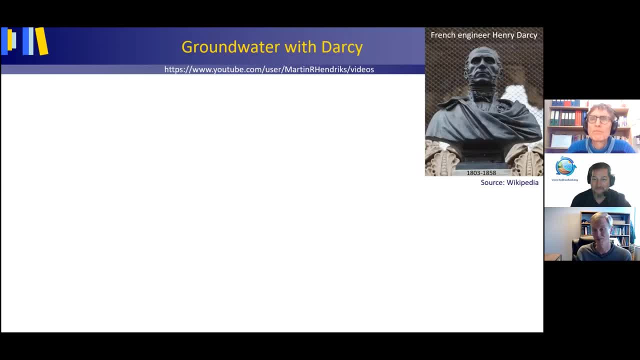 is whether water will flow back into the pit or will it be a flow-through pit where it will just continue to flow through, like Martin showed in his example, and it would continue to go to the discharge point, which is a river? You assess that typically? 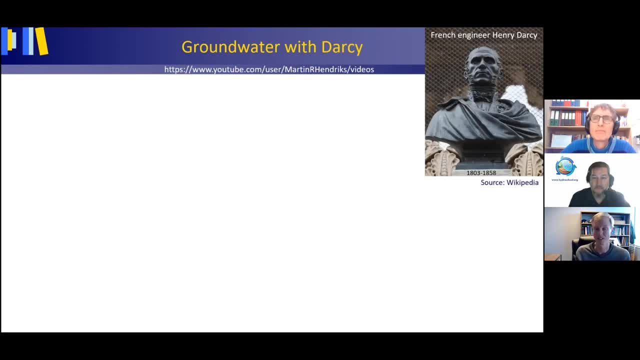 through predictive numerical modeling and kind of calculate a new quasi-stick model of a new quasi-steady state once you've stopped mining, and look at the recovery periods. So yeah, it's very applicable- the first principles that Martin's talking about- to mining as well. 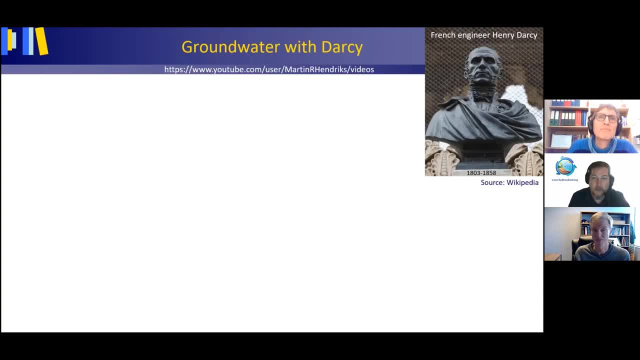 Yeah, And so thanks for those questions. So again, one of the questions was on groundwater surface water interactions. We'll talk about that a little bit more, but a lot of these same principles in this very beginning part if you watch some of our introductory lectures. 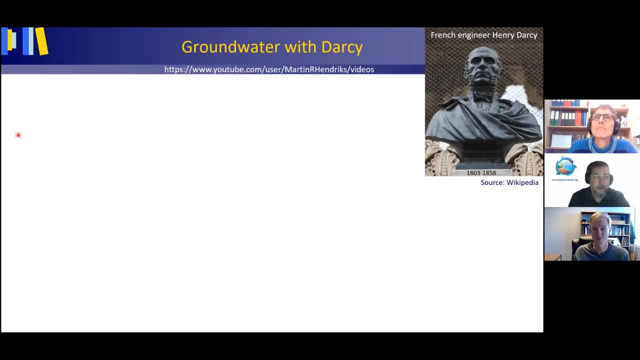 on some of those others: Euler and Bernoulli- we hit those with our surface water course. We also hit Froude and Manning and others, because we've got full webinars covering some of the theory and practical applications that came from some of those other. 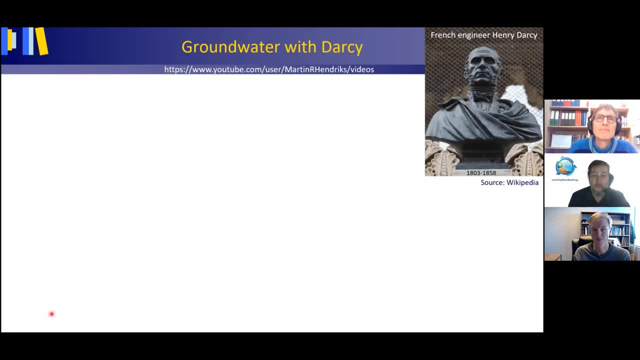 well-known names in surface water, And Bernoulli is one that applies to both. Darcy, on the other hand, which we'll talk about now, is generally somebody that we talk about in terms of groundwater- primarily in groundwater, but we'll see. 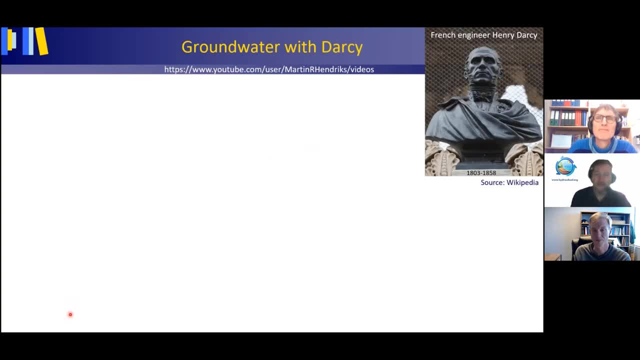 if there's some interaction there as well. So back over to you, Dr Henderson. Okay, Thanks, Gray. Moving on to Darcy's law, we again start off with a little quiz, As far as I know, especially for all those. 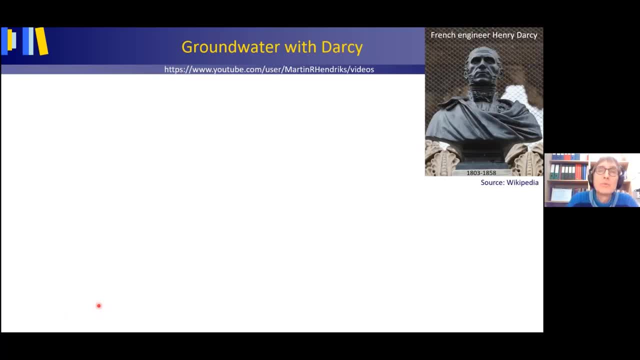 already familiar or slightly familiar with hydrology, with groundwater hydrology, which one of the following sentences presents a correct calculation method. There is only one correct calculation method. A: the hydraulic conductivity is one centimeter per day, then groundwater travels one meter in 100 days. 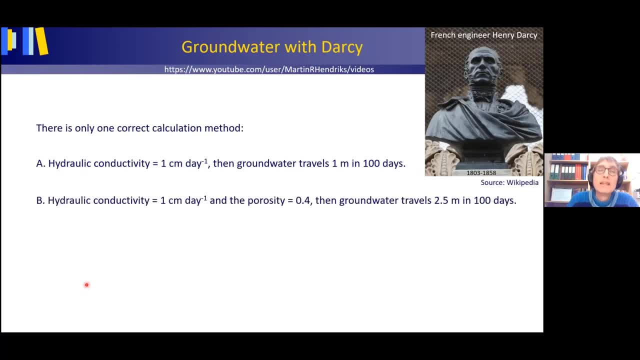 Or is it B? the hydraulic conductivity is one centimeter per day and the porosity, which is the maximum volume fraction of water in the subsurface, is 0.4, then groundwater travels 2.5 meter in 100 days. 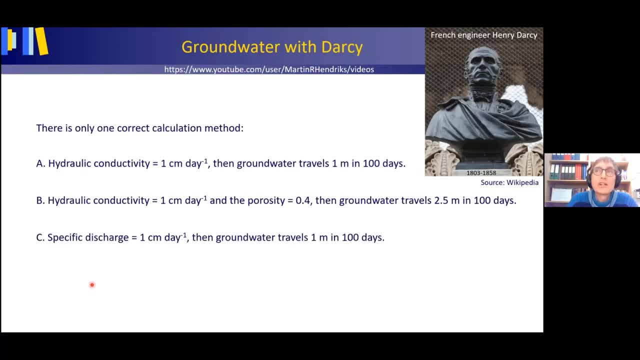 Or is it C? the specific discharge is one centimeter per day, then groundwater travels one meter in 100 days days. or is it D? the specific discharge is one centimeter per day and the porosity is 0.4, then groundwater travels two and a half meter in 100 days. There is only one right option. 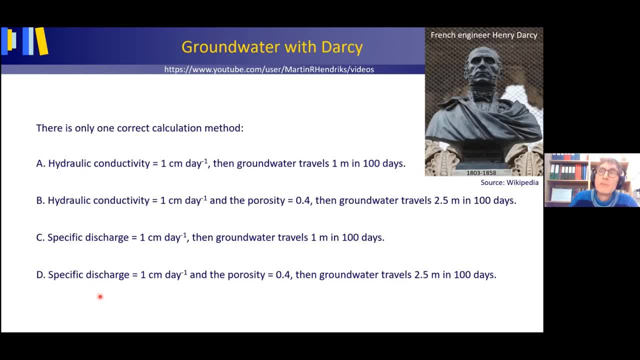 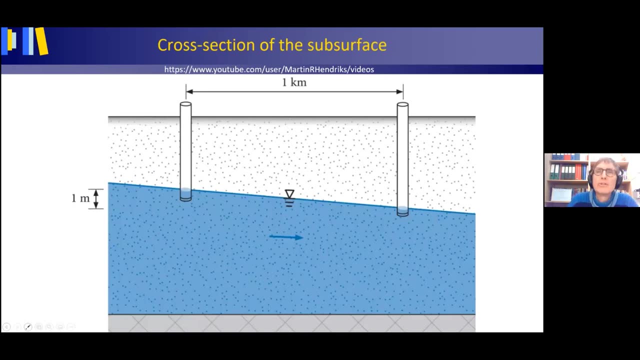 which option presents the correct calculation method. If you like, write down the letter of your choice and check later whether it's correct at the end of this lecture. Here we have the cross-section of the subsurface of a flat land surface. We have the land surface, the subsurface. 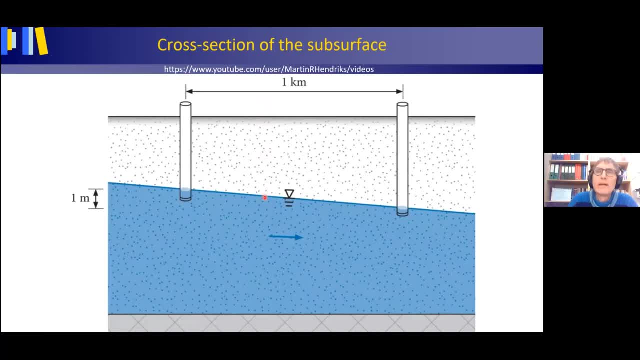 is made up of well-sorted sand. we have the water table and groundwater above an. a water impermeable layer Installed into the subsurface are two water panels and two water panels and two water panels And, as said before, groundwater can only enter the piezometer tubes through the screens at the bottom. 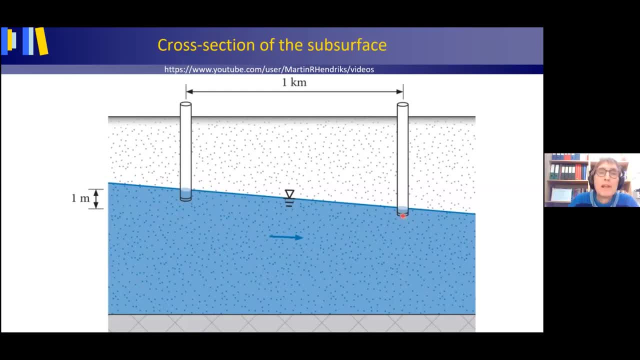 Taking the top of the water impermeable layer as a reference level, we see that the water rises to a lower level in the right piezometer. The right piezometer thus has the lower hydraulic head and groundwater flows in the direction of the lower hydraulic head, thus from left to right. 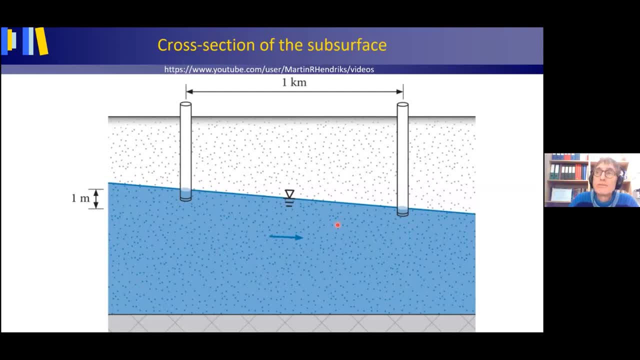 Can we estimate the velocity of the groundwater flow? If yes, we can also establish the time it takes for a conservative pollutant at the left piezometer screen to reach the right piezometer screen. A conservative pollutant is a pollutant that does not interact with the ground mass, or in other words, the polluting substance goes with the flow. 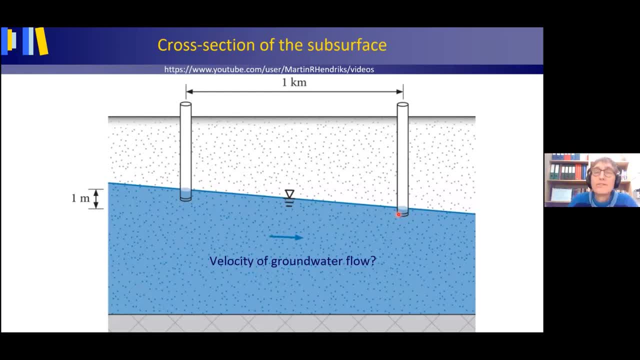 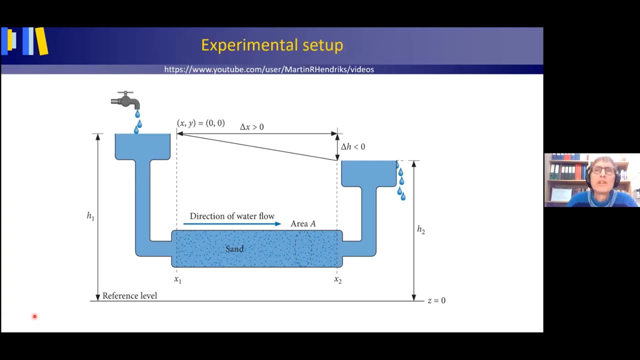 Again, can we estimate the velocity of the groundwater flow? Yes, we can, and for this we can make good use of Darcy's law. In his original experiments, Darcy used a vertical cylinder filled with water-saturated sand. Darcy's experimental set-up is represented here in simplified form by a horizontal cylinder filled with water-saturated sand. 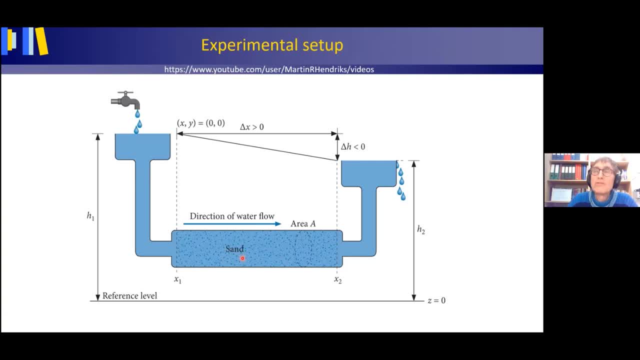 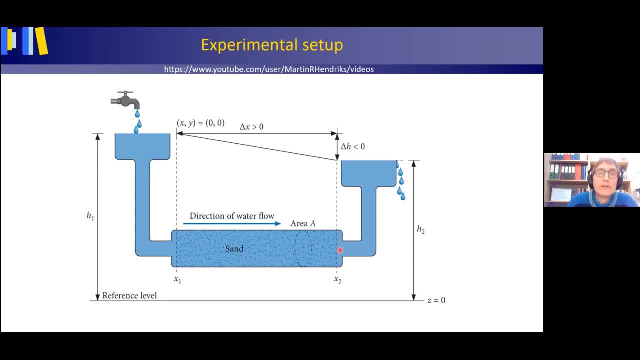 and the water flow has become steady, or another word for this stationary. the volume, flux Q or discharge Q, which is the volume of water that moves through any vertical area A per unit of time, in cubic meter per day, can simply be measured by collecting the water that spills over the receiving reservoir during a fixed time interval. 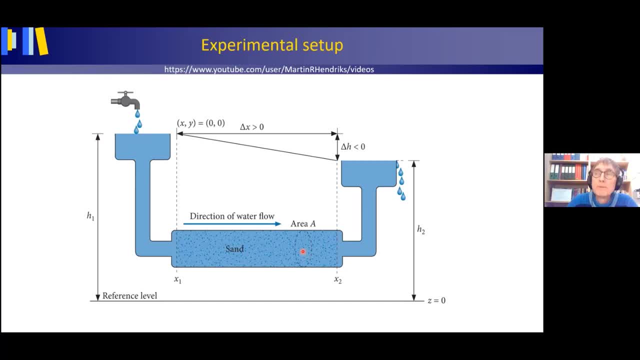 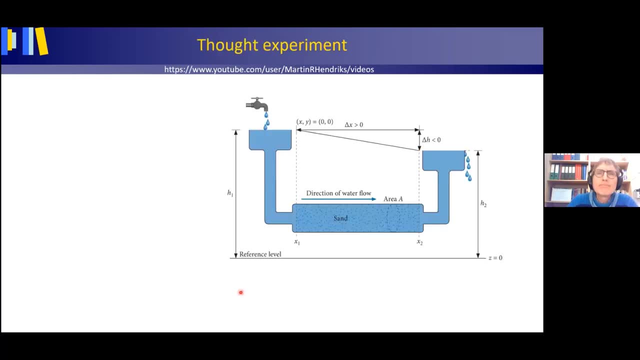 Note that the area A is perpendicular to the water flow. Let's do a thought experiment. What would happen if we would enlarge the difference between the hydraulic heads H1 and H2?? For this we could raise the left reservoir to a new, fixed, higher position. 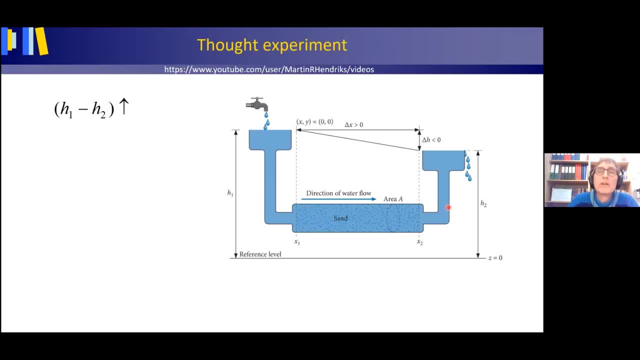 or lower the right reservoir to a new fixed lower position, or do both Intuitively. you would think that the volume, flux or, another word for this, the discharge in cubic meter per day would increase. So when H minus H2 increases, 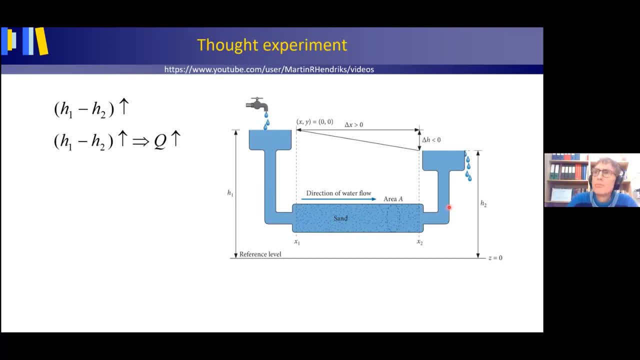 Q increases. What would happen if we would diminish the distance X2 minus X1? The length of the porous medium resisting the water flow then diminishes and the discharge would most likely increase. So when X minus X2 minus X1 decreases. 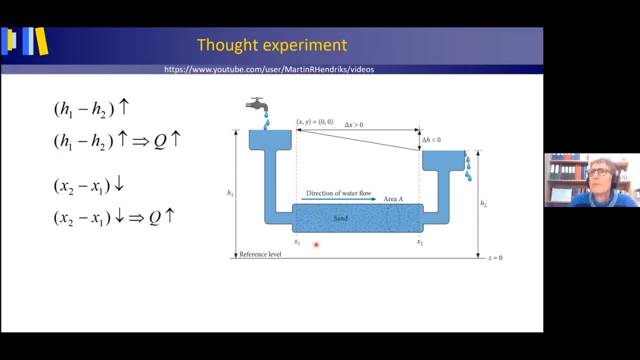 Q increases. What would happen if we would enlarge the distance between the hydraulic heads H1 and H2?? What would happen if we would enlarge the area A of the cylinder perpendicular to the flow? Then we would also enlarge the pores within this area A, through which the water flow actually takes place. 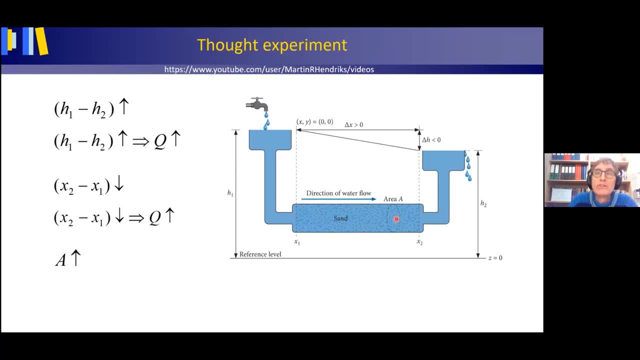 And the discharge would increase. So when A increases, Q increases. Importantly, please already know that groundwater flow is through the pores and not through the solid surface. We can now already establish part of Darcy's law. The volume, flux or discharge Q through the porous sand material is linearly related to both the difference in hydraulic heads, H1 minus H2,. 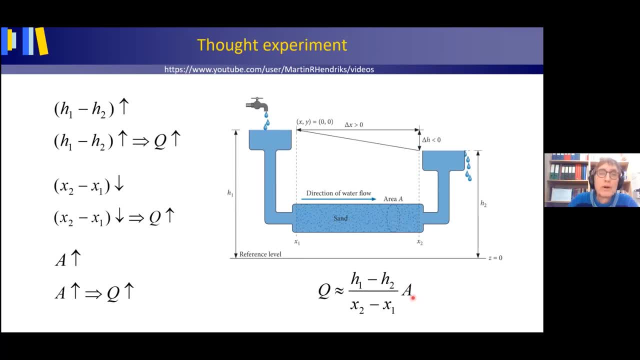 and the area perpendicular to the groundwater flow and inversely, linearly related to the distance of flow through the porous material: X2 minus X1.. Here we have the relation again, but it's not looking very neat because here I have a term with 1 minus 2,. 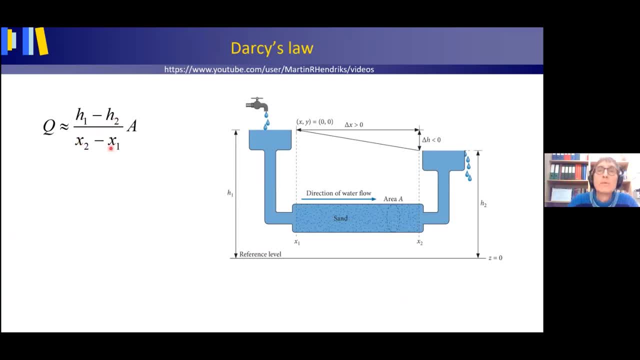 and here it's the other way around. The difference in hydraulic head delta H over the cylinder length is defined as the hydraulic head at the water receiving end- H2,, minus the hydraulic head at the water dispatching end, H1, and not the other way around. 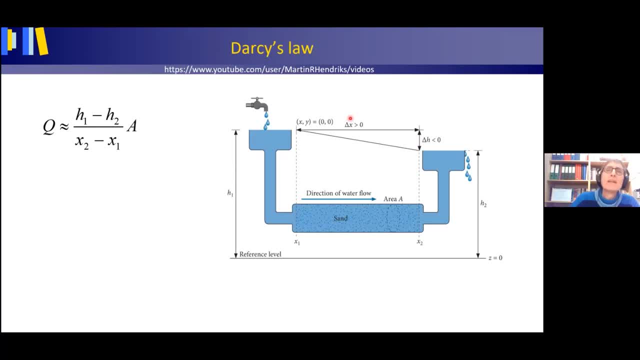 The distance delta X is defined as the location to which water flows- X2, minus the location from where it was dispatched- X1,- and not the other way around. For this horizontal water flow, the distance delta X thus equals X2 minus X1. 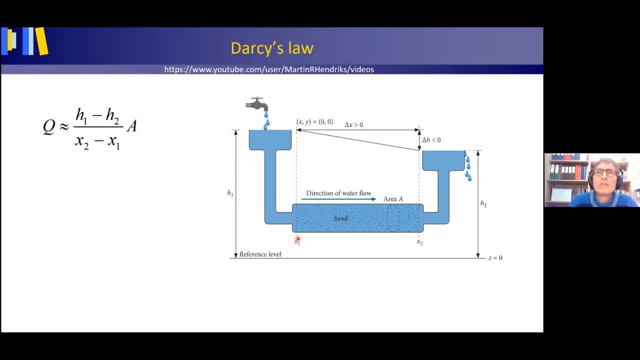 Following these definitions, we can now rewrite the relation as Q being related to H2 minus H1, divided by X2 minus X1, and this times A, But now, of course, with a minus sign added to the equation: The hydraulic gradient. 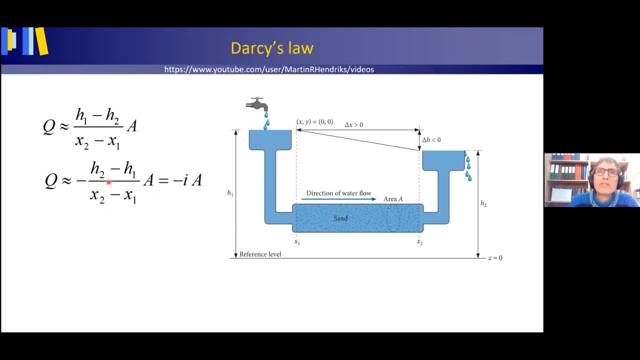 is defined as the difference in hydraulic head H2 minus H1, over the porous medium divided by the distance. sorry, as the difference in hydraulic head H2 minus H1, over the porous medium divided by the distance X2 minus X1,. 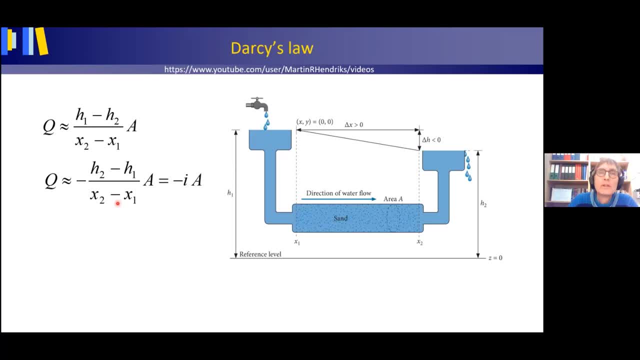 over which this difference in hydraulic head occurs. The hydraulic head is given here as a small i, So Q equals minus the hydraulic gradient. I times the area perpendicular to the water flow Again, regard this area A as a kind of false area. 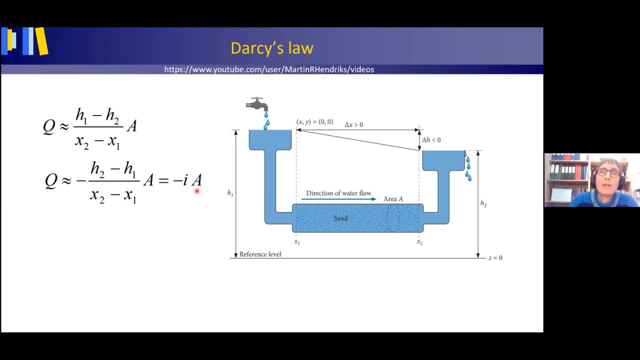 as ground water flow is not through the area in full but only through the pore space part of the area, not through the solid part made up by the sand particles, But still the equation is not looking very neat To the left of the 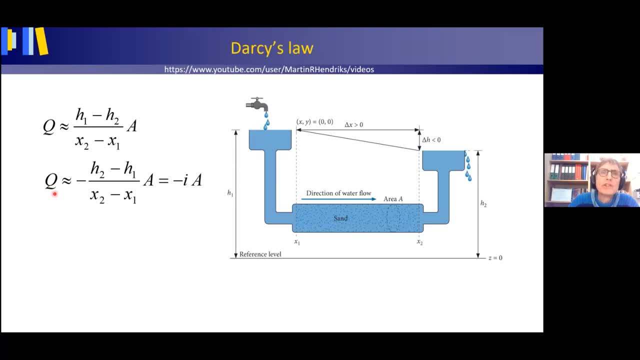 equal sign, the volume, flux or discharge Q is in cubic meter per day And to the right of the equal sign the hydraulic gradient is in meter per meter, so dimensionless, And the area A is in square meter, So we have cubic meter per day. to the left, 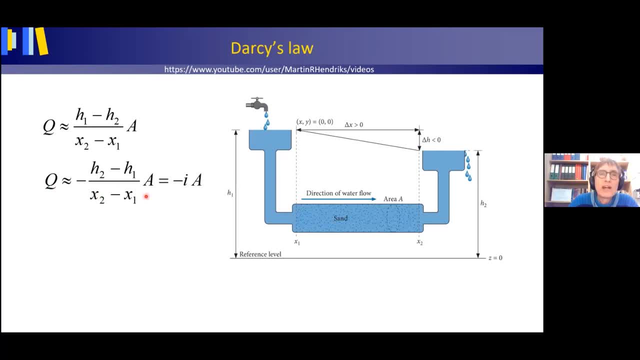 and square meter to the right of the equal sign And thus we are still missing out on a term in meter per day to the right. This term is the hydraulic conductivity K in meter per day. The hydraulic conductivity is a function of both the properties of the porous medium. 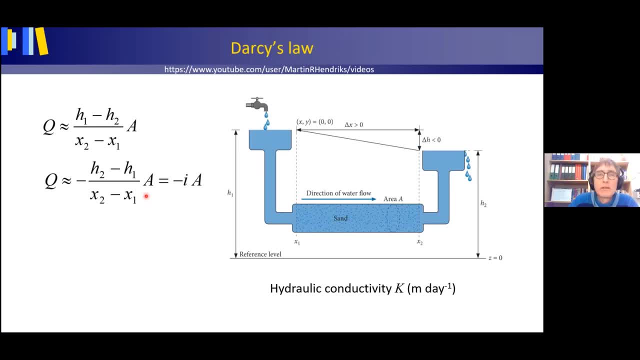 through which the water flows, and the properties of the water itself. Without going into full detail concerning the properties of the porous material, think of: is it sand, loam, clay or a mix of these? Is the material well-suited? 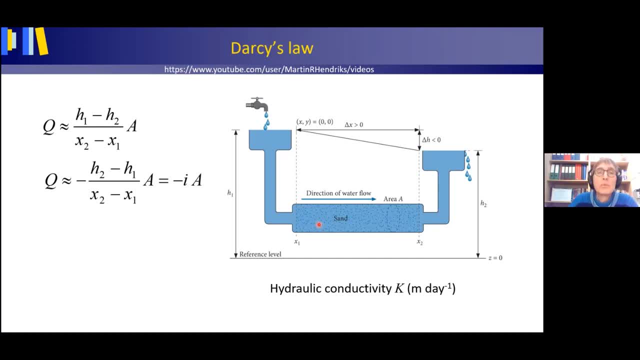 Or not. For instance, a well-suited sand will have a much higher hydraulic conductivity than a clay. Concerning the properties of the water, think of its temperature, density and viscosity, For instance. the hydraulic conductivity increases when the water temperature rises. 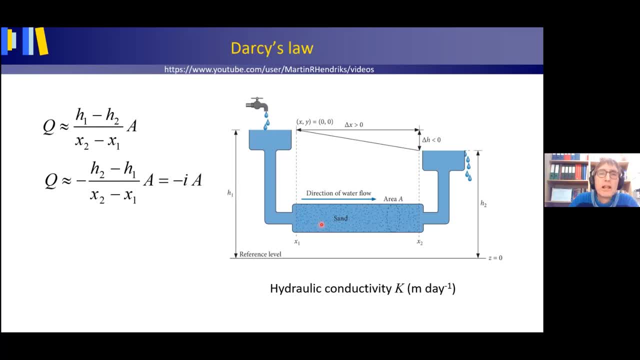 All these properties of both the porous material and the groundwater itself are captured in this hydraulic conductivity K. Our thought experiment, has replaced part of the experiments and observations that led Henri Darcy to his law, which is what we now have deduced: The volume flux. 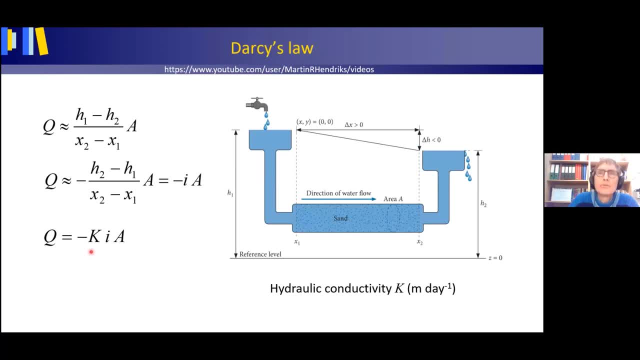 or discharge. large Q is equal to the minus K times I times A. However, if you look at literature, you usually find Darcy's law expressed as: small Q equals equals minus K times your hydraulic gradient I, Instead of using small I. 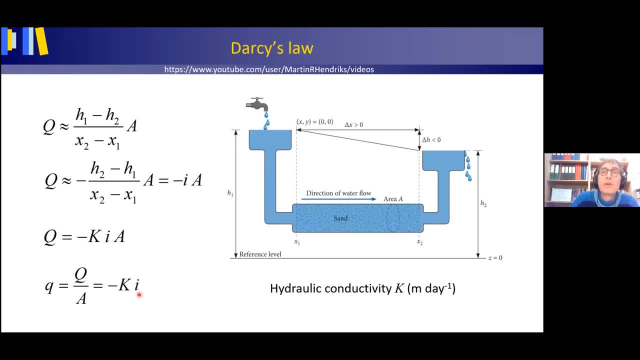 the hydraulic gradient for horizontal groundwater flow in literature is also given as delta H over delta X or sometimes as the differential dH- dx. Small Q is large Q divided by the area A perpendicular to the flow and thus in meter per day. Small Q in meter per day. 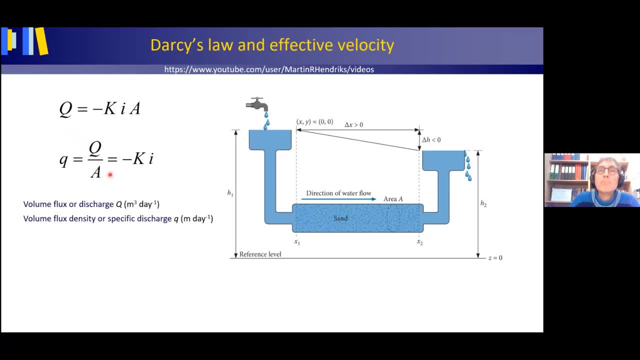 may be mistaken for a velocity, but remember that groundwater flow is only through the pores of area A and not through the area A in full. Therefore, small Q, despite its unit of meter per day, is not a velocity. We call small Q 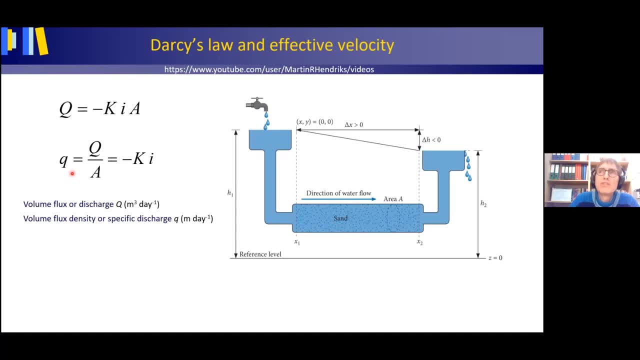 the volume, flux, density or the specific discharge of the groundwater flow. If we want to know the true velocity of the groundwater flowing from X1 to X2, of course we need to know the porosity, Actually the effective porosity. The porosity is usually indicated with 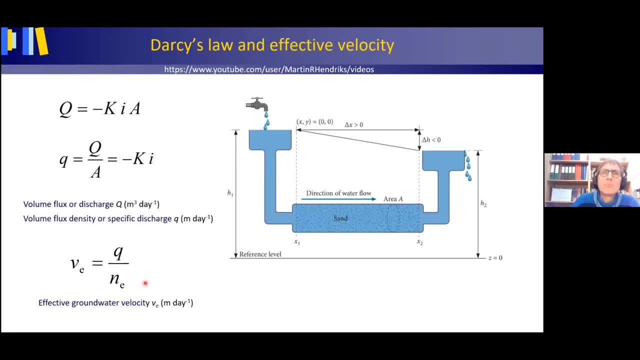 small n and is defined as the maximum volume fraction of water in a porous mixture. A volume fraction is expressed as a number between 0 and 1.. As there, for instance, may be stagnating water in dead-end pores in the porous material, 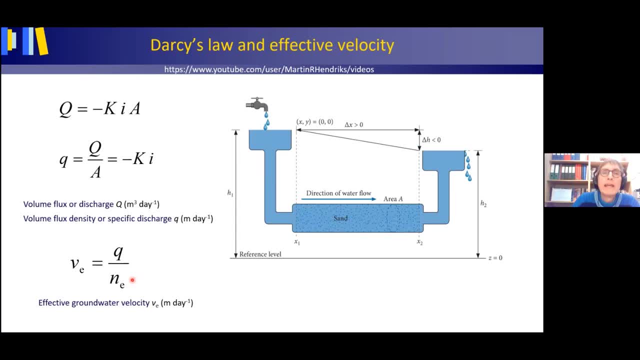 the effective porosity and with subscript E, is defined as the volume fraction of the porous material that participates in the groundwater flow process. As only the pore space within the area A participates in the groundwater flow, this true velocity, which we call the effective groundwater velocity. 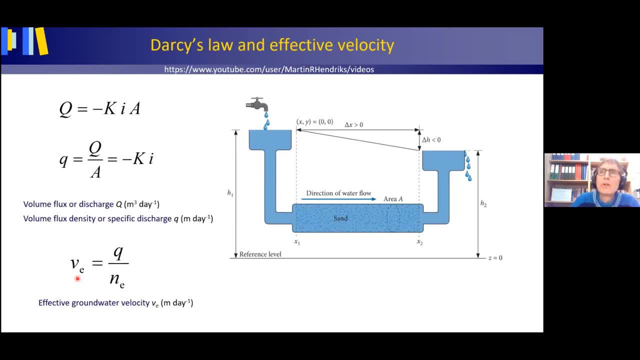 B with subscript E must be equal to the volume density, the volume flux density or specific discharge small q divided by the effective porosity. Also, if we were to inject a colouring dye at the left screen here, we could easily estimate the time. 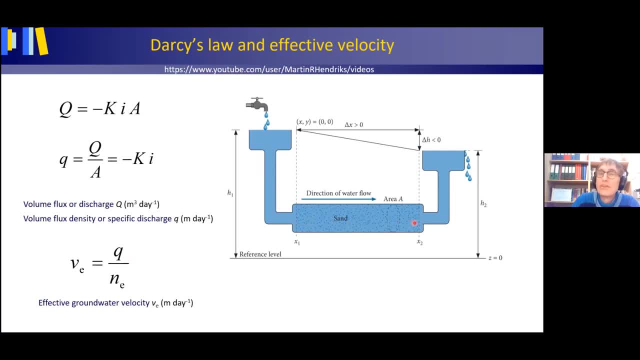 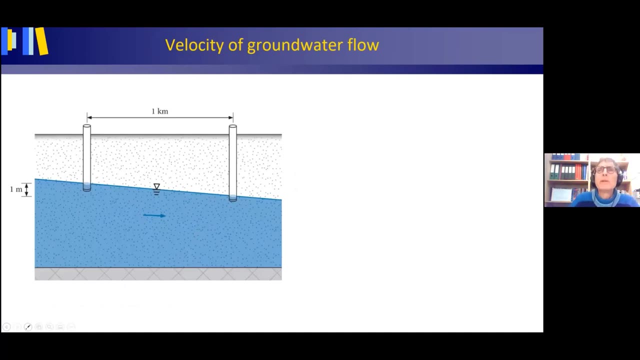 it would take for this colouring dye to reach the right screen simply as the distance, x2 minus x1, divided by this effective velocity. Let's return to our problem. Can we estimate the velocity of the groundwater flow? As said before, yes, we can. 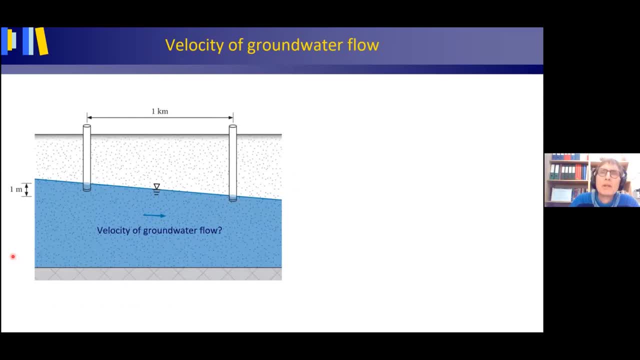 but for this we need some extra data. The subsurface is made up of well-sorted sand. The hydraulic conductivity k will then be in the order of, let's say, 10 m per day. We know the difference in hydraulic head to be defined as the lower hydraulic head. 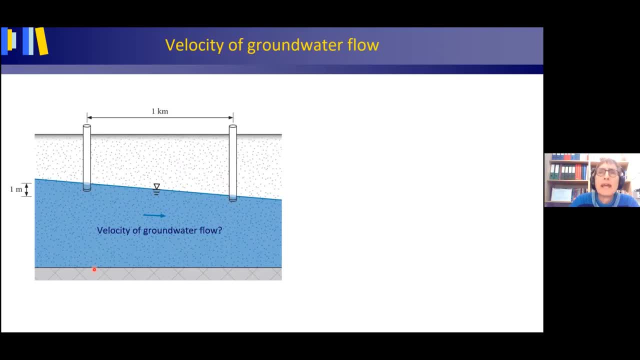 minus the higher hydraulic head, thus minus 1 m here, and this difference in hydraulic head is established over a distance of 1 km. Hydraulic gradient for this phreatic or unconfined water flow may then be taken as this: minus 1 m divided by 1000 m. 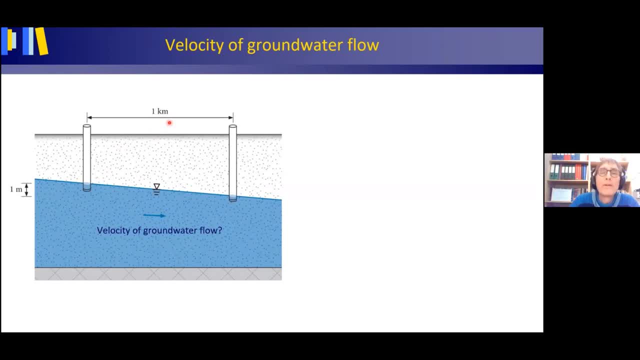 which is 0.001.. Using Darcy's law, the volume, flux, density or specific discharge, small q equals minus k times I the hydraulic gradient. so minus 10 times I, times minus 10 to the power minus 3,. 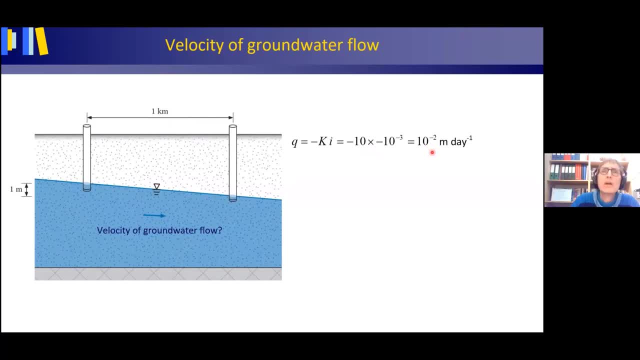 which gives 10 to the power, minus 2 m per day, which is 1 cm per day. This, of course, is not yet the velocity. To determine the effective velocity, we need to know the effective porosity Ne of the well-sorted sand. 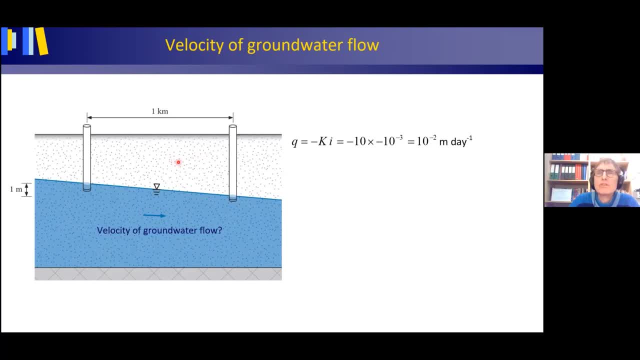 Ne of the well-sorted sand can be in the order of 0.4.. The effective velocity is small: q divided by Ne, which gives 10 to the power, minus 2 divided by 0.4,, which gives 2.5 cm per day. 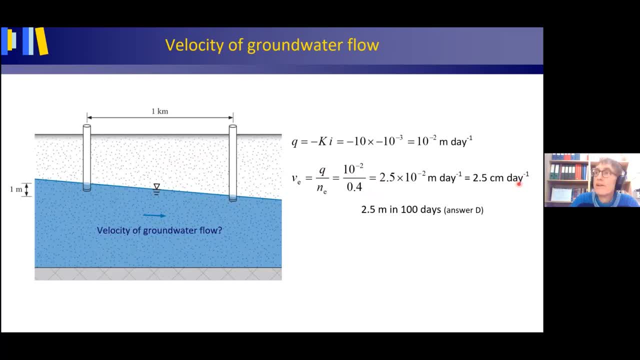 which is 2.5 m in 100 days. So answer D of the earlier multiple choice question: For a correct calculation method you always need to know the porosity, or better, the effective porosity, which was unknown in the earlier multiple choice options A and C. 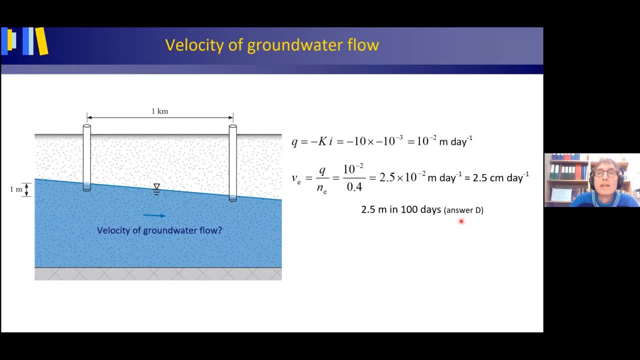 Plus, you need to know the hydraulic gradient, which is incorporated in the specific discharge but not in the hydraulic conductivity, thereby discarding the earlier multiple choice option. B 2.5 m in 100 days is 9 m per year. 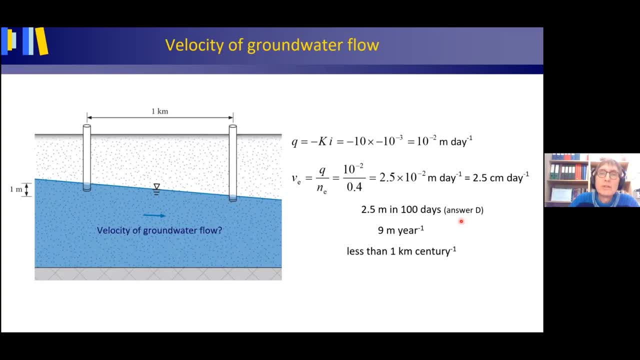 which is less than a km in a century. Actually, the time it takes for a conservative pollutant at the left piezometer screen to reach the right piezometer screen is equal to the distance of 1000 m divided by 2.5 times 10, to the power minus 2 m per day. 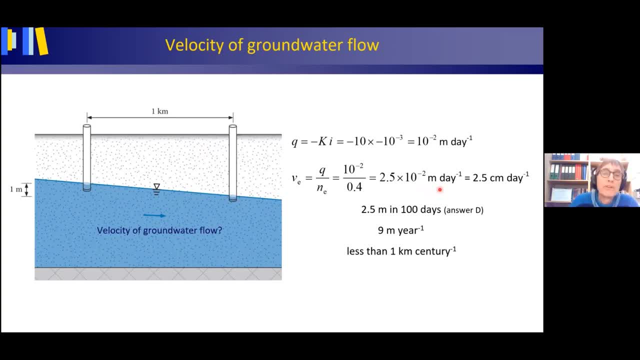 which gives 40,000 days, or more than 109 years, And less than 1 km in a century, amounts to a mere stretch of 10 km in 1100 years. Thus groundwater, with some exceptions, for instance in karst areas or when pumped. 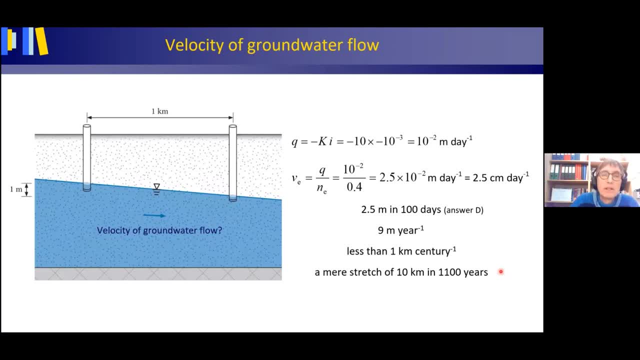 flows very slowly And the energy related to the water's velocity, the kinetic energy, therefore did not need to be considered earlier when using Bernoulli's law for groundwater flow As a side remark in surface water flow, which is rapid flow and may even be turbulent. 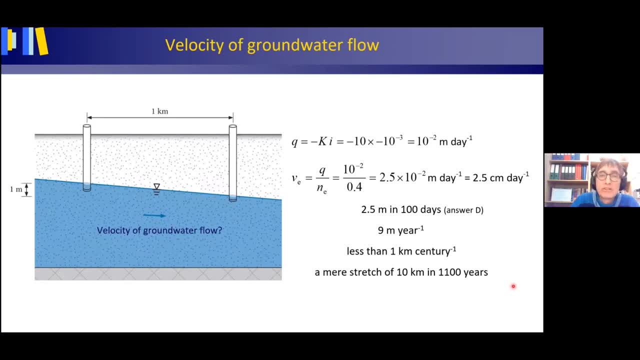 evidently, the kinetic energy does need to be considered and can then, in a similar fashion as with the other energy terms shown before, be rewritten to a length unit called the velocity head. To finalize, we have observed that unconfined groundwater can flow along curved pathways. 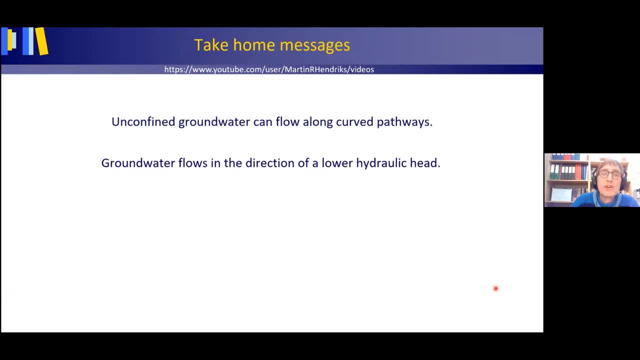 We know that groundwater flows in the direction of a lower total energy, a lower hydraulic head, And thirdly, as just deduced, groundwater generally flows very slowly, Also the minus sign in Darcy's law, as well as the differences between specific discharge. 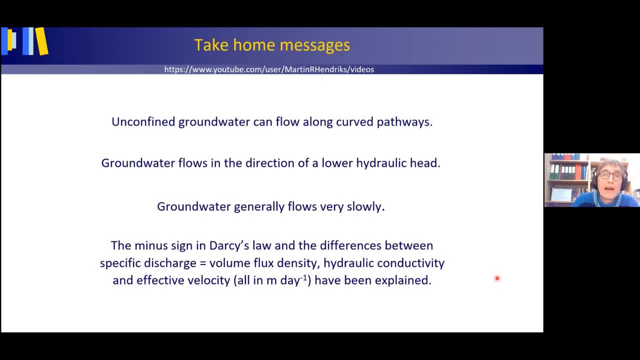 being a volume, flux, density, and the hydraulic conductivity and the effective velocity, all in units of m per day, have been explained. This lecture introduced groundwater hydrology, so there is much more Very important in mastering hydrology, in mastering groundwater hydrology. 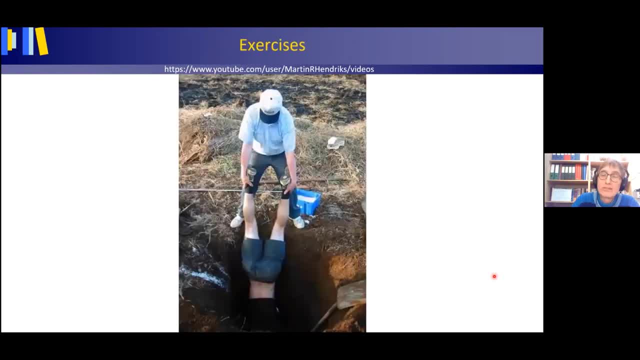 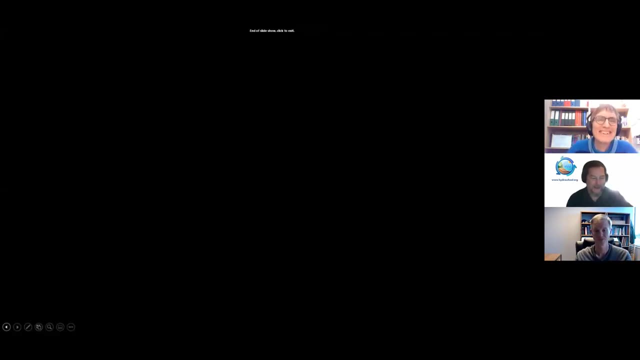 is that you have to struggle with exercises. I wish you success with all your future hydrological endeavors, And that's the end of part two. Great, And we might have some advice about entering confined spaces here. Now we've got about 10 minutes to go. 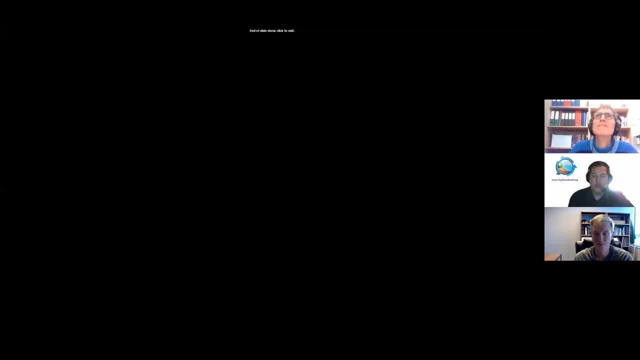 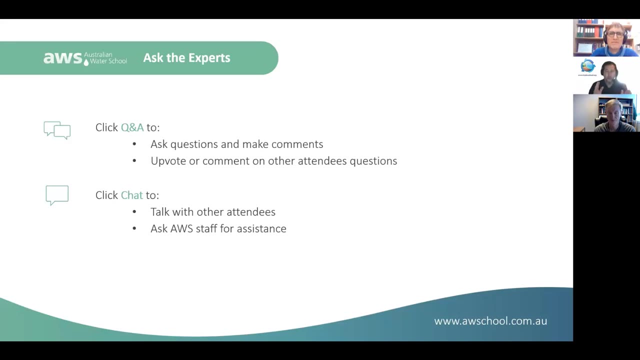 Thanks so much for that, Dr Hendrix. Again, what happens here when we go back to basics? hopefully, when you go all the way back to basics, there may be some things that are very clear to you. What we generally find is: 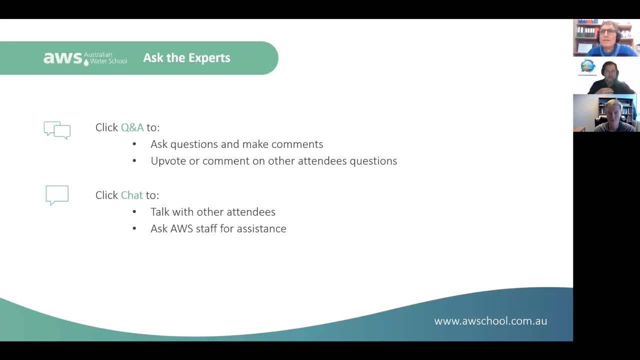 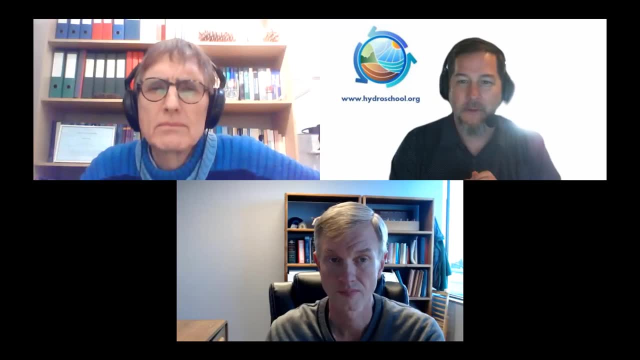 at some point we lose it. We'll keep up, we'll keep up and we'll say, okay, I've got that, I've got that, I've got that, and then the lecture or the class gets ahead of you. 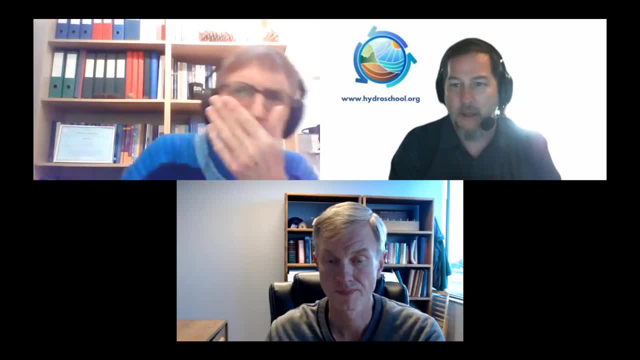 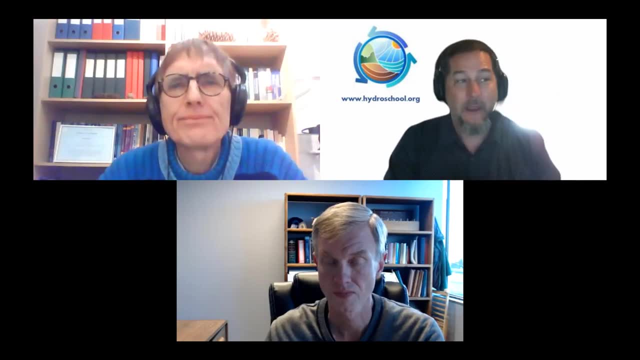 and you've got to go back and figure things out, And that's the whole point. when we come in and do this Groundwater Essentials course, We want to make sure that everybody keeps up, and then, when we get to certain points, there will be exercises where you've got to practice it. 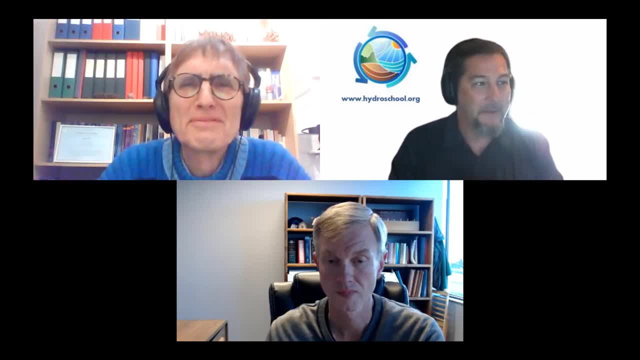 and you've got to demonstrate that you're keeping up with these concepts to be able to get into the next one, Because once you get behind and the lecture starts going over your head, you may as well just stop and try and figure it out from there. 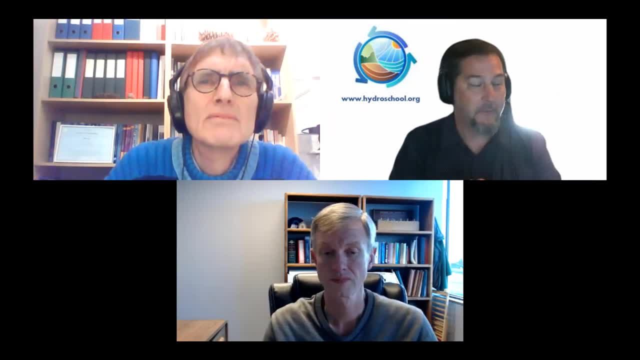 So I hope you've got to feel a little bit for how these courses are going to proceed as we go forward in March, But also in the meantime let's have a look at some of these questions that have come in on the Q&A line. 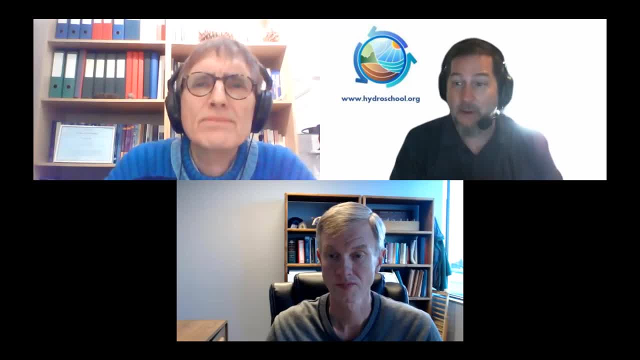 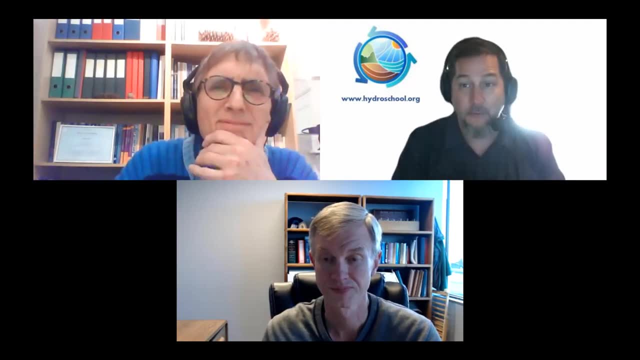 Now Guy has frantically been answering some questions there. There have been some great questions. Let's start with just one that relates to the surface water people who are on board. We've got about a third in each category, according to the poll results. 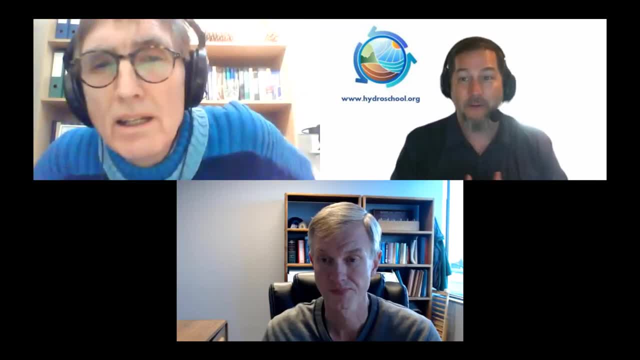 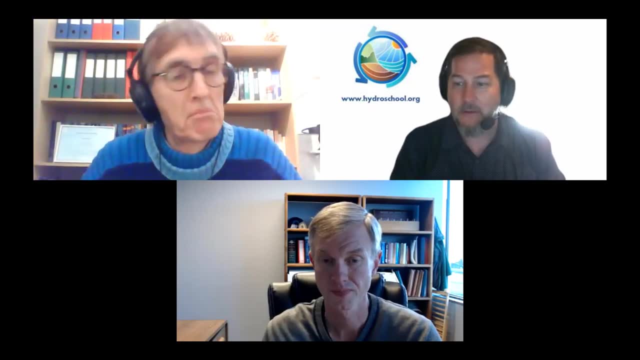 So one that would apply to everybody is: when can friction be ignored? We talked about that in the very beginning. Hey, let's ignore friction and move into this. Guy, I think you had an answer on that one. Anything you wanted to share with the audience on that response? 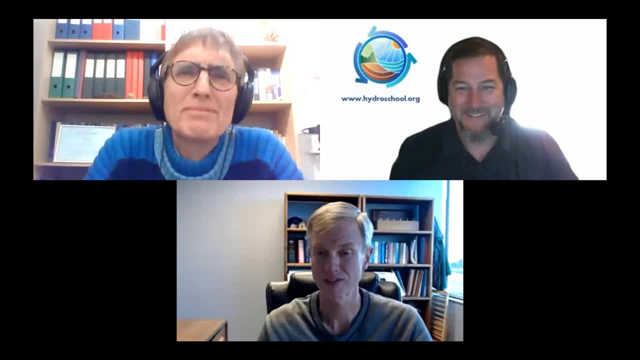 Well, the actual question was: is there an example where friction loss is zero? Yes, And I couldn't think of one off the top of my head, So maybe if Martin can think of one, But yeah, there's clearly always in real life. 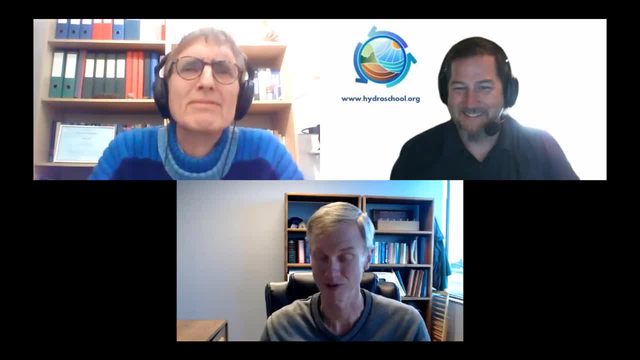 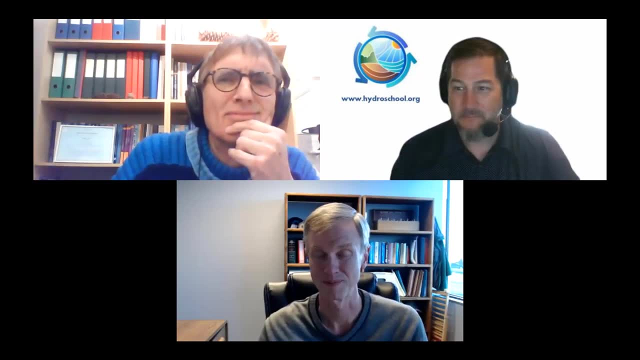 there's going to be friction between the water molecules at the molecular level. There's going to be friction between the water hitting pores, you know, in the force media. So yeah, But I can't think of an example where it's zero. 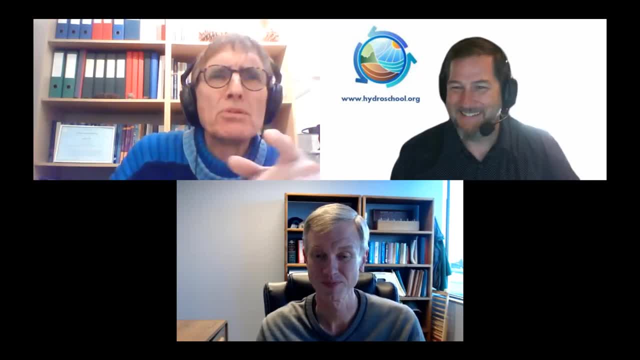 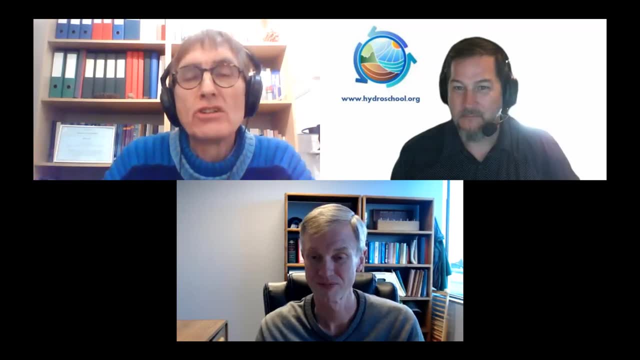 Now, this is the typical difference between reality and a model. In reality there is friction, But very often we say there is no friction. also in surface water hydrology. And when you say there is no friction, you can say that the total energy at two different points. 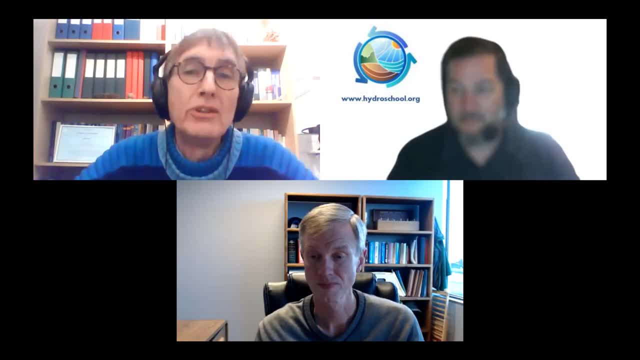 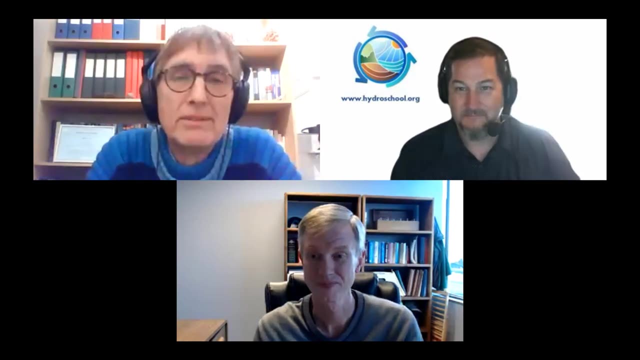 which are not that far apart is the same And you can make calculations based on that. So that's very common. That's very common in surface water hydrology And well, in groundwater hydrology maybe. yeah, there's a difference between reality and the model. also, 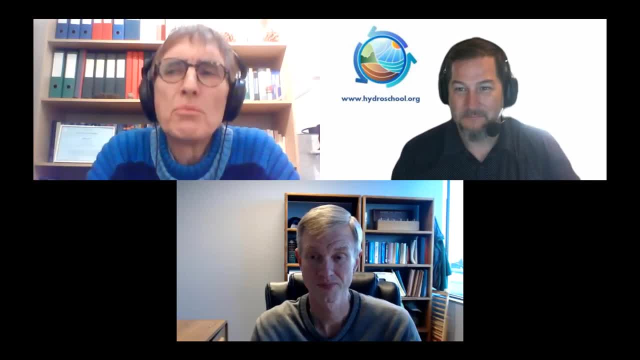 But usually the assumptions we make in our model they are quite sound And the answers are not far off. Yeah, And especially in a numerical model, if you have a very fine network, then you can really come to good answers. By the way, in the course, 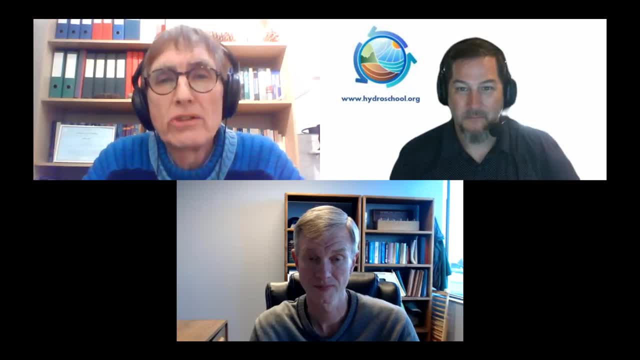 we'll be dealing with kind of groundwater hydraulics, analytical groundwater hydrology, And that's especially valuable, as analytical groundwater hydrology gives you easy methods to make a kind of crude calculation. So then you know in what kind of order your outcome from your numerical model should lie. 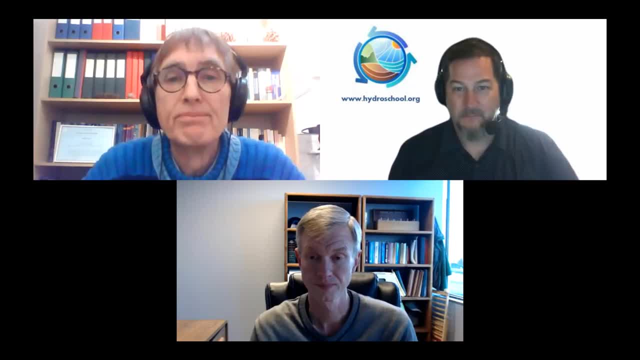 It's very important, especially in that sense. Yeah, And one of the things we want to do is take away the mystery of the black box. That's what we try to do in our surface water course with, like Manning's coefficients and things like that. 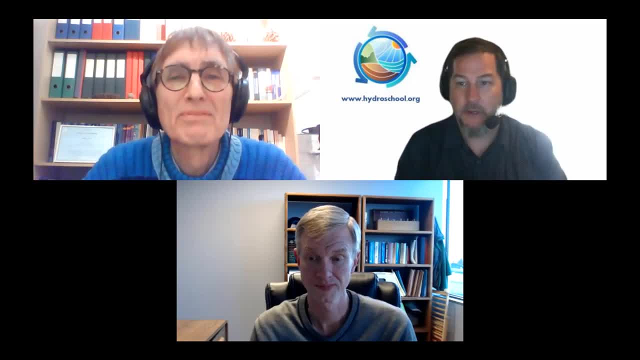 So the K value. we hope, with lectures like this, that when you start plugging things into models, the porosity or whatever else you're plugging in, that there's an understanding of where that comes from and how it figures into the equations. 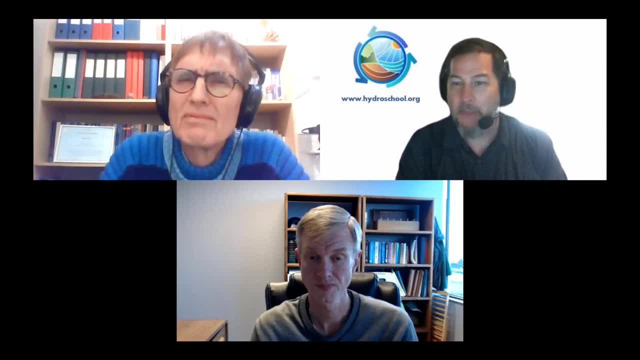 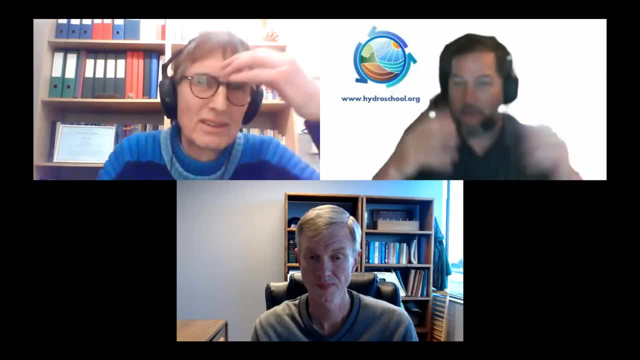 Now somebody had a pretty intuitive question here, Martin. when you put up that picture of the piezometer and you said it's only screened from the bottom, then somebody asked the question: well, what if it was screened all the way? 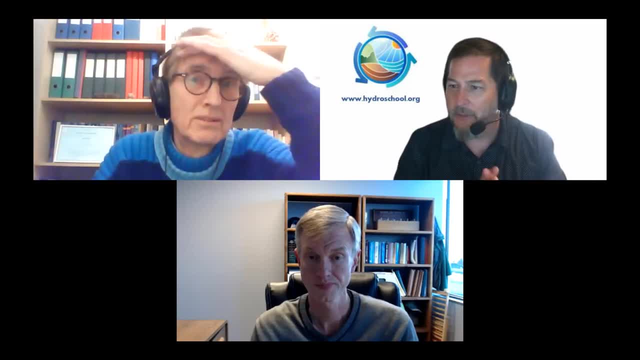 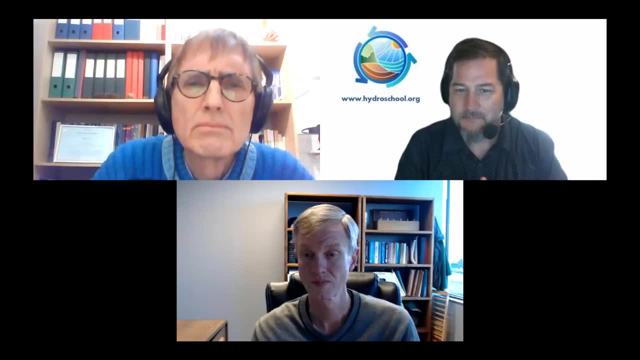 What if you perforated the entire thing? Guy, you had an answer to that one as well in the chat line, So, Guy, maybe just state your answer and then, Martin, you can follow up on that. Yeah, Yeah, I think they were talking about. yeah. 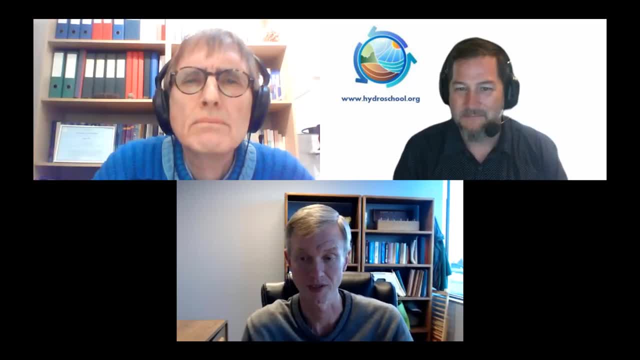 full length screen in the confined aquifer versus one just screened over the top. And I was just talking about the difference between partial penetrating wells and fully penetrating wells. And typically partial penetrating well, you'll induce more drawdown in the aquifer. 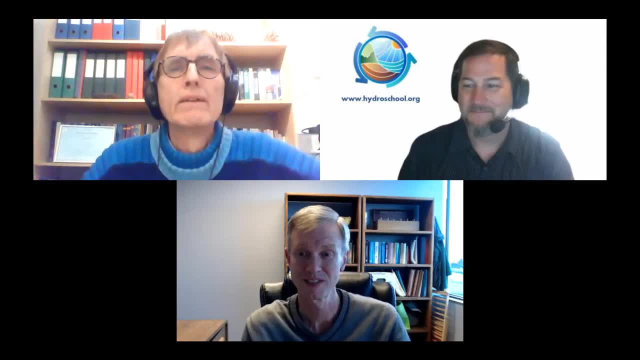 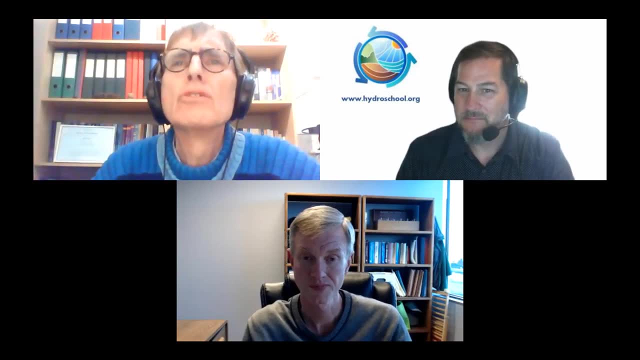 was what my answer was. But go ahead, Martin. Yeah, that's true. Maybe some people have also noticed that in the first part of my talk I have a picture here. Can I start sharing? You can start sharing again and put it back up. 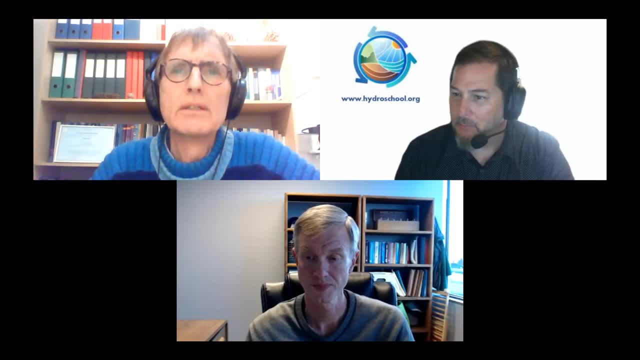 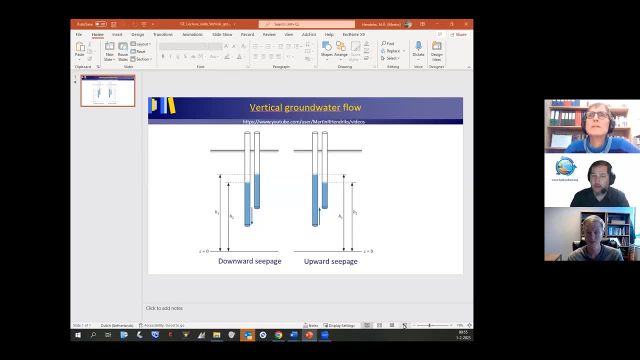 if you've got that, Where is? yeah, While we're doing that, I've also mentioned then that, if you are interested in groundwater contaminant transport- so we did talk about those plumes going through- we're going to have this. next course is going to be handling. 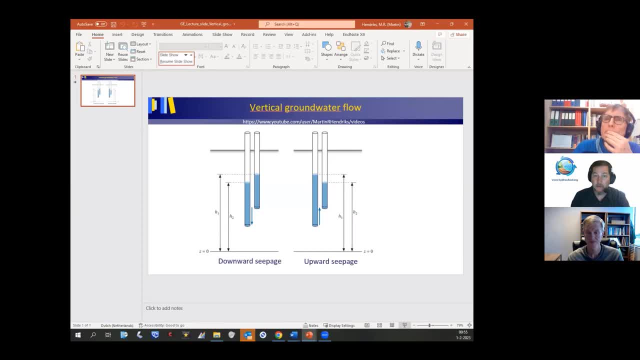 groundwater, hydrology and hydraulics. Later on in this year we're going to follow up with full water quality essentials courses in both surface water and groundwater, So if you're interested in contaminants, stay tuned. It won't be part of this March course. 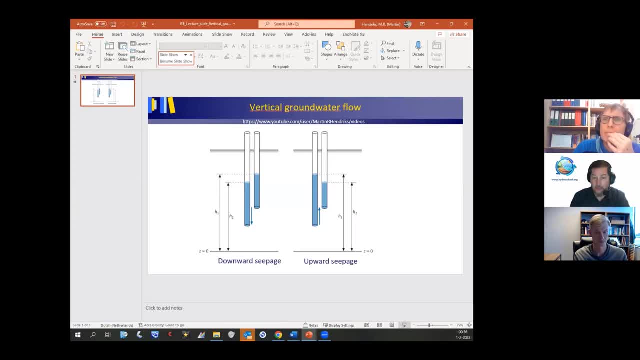 but we are going to cover that in the future, So I can see your picture now. if you want to talk to that one, Yeah. but to continue what Guy was saying, the difference between partial penetrating canal, then you get these curved flow lines. 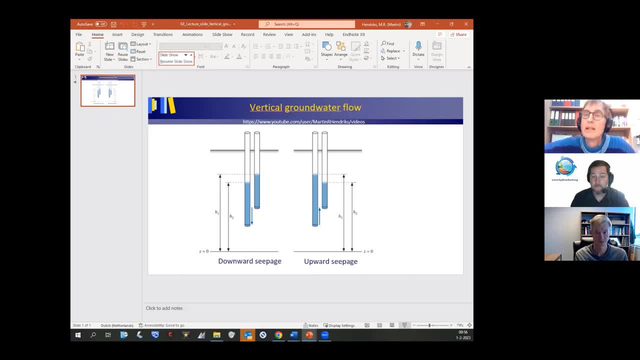 If you have a fully penetrating canal, which is a canal which goes all the way to the lower lying water impermeable layer, then your groundwater flow becomes more horizontal. So maybe some people have also noticed that at the beginning of my talk I had a curved water table in part one. 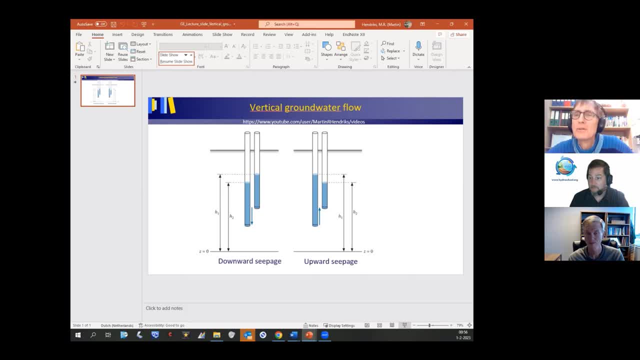 and in part two, my water table was quite straight, which is actually a kind of, which is not totally truthful, because there it is also curved, but we can make our calculations as if that groundwater flow is horizontal. But to come back to the question of 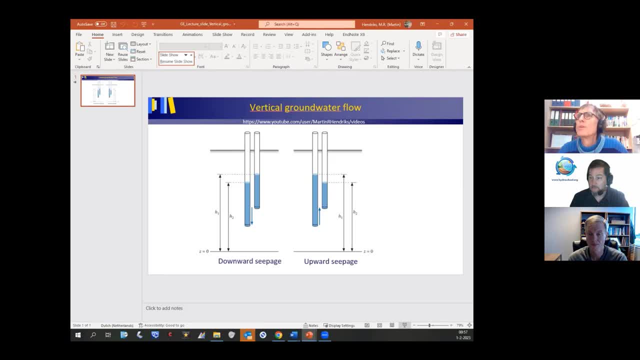 what if the whole tube was perforated? then you would measure the water table actually. So you can see, for instance, in this right picture, which is a common picture in the Dutch polder where I live, if you have your screen deeper down. 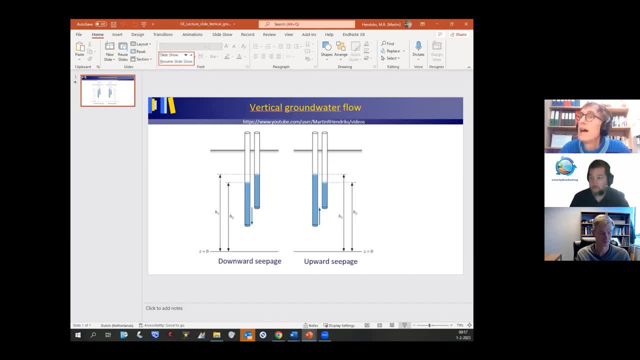 you have a higher hydraulic head than when your screen is higher up, So water is flowing upwards, And in the recharge area you have the opposite, where you have the higher hydraulic head here and the lower hydraulic head here. Now where would the water table be? 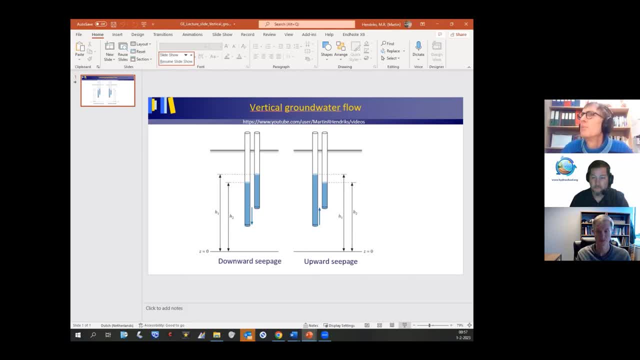 The water table here would probably be, because if I put my screen here I would find an even lower position because water is moving upwards. So the water table would probably be somewhere here. You can measure the water table if you put your pitometer screen. 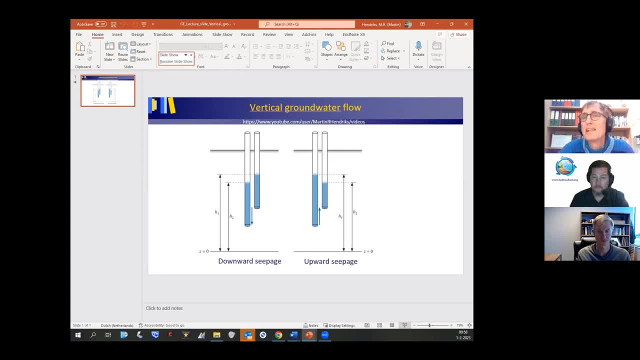 exactly at the position where the water table is, But that is, of course, a bit ridiculous. The more common way to measure it is to have a tube which is perforated all the way down, So it's one big screen in reality. 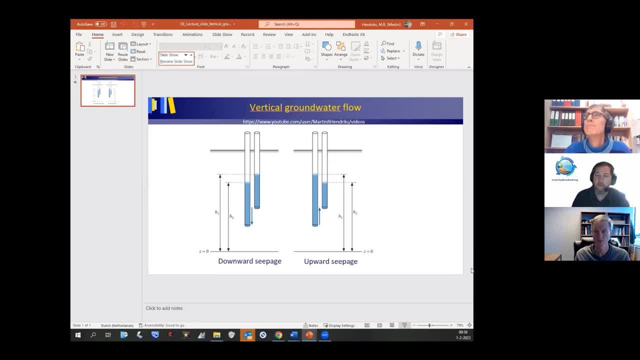 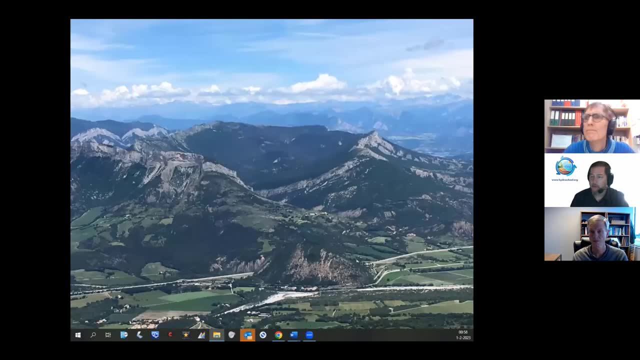 Excellent. Maybe one final question: Just get your comments on some of the discussion that went back and forth on the Q&A line dealt with the confined versus unconfined aquifers and how you could tell Now with that picture you had up there. 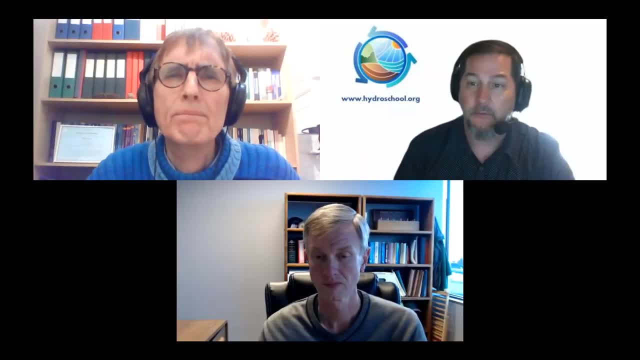 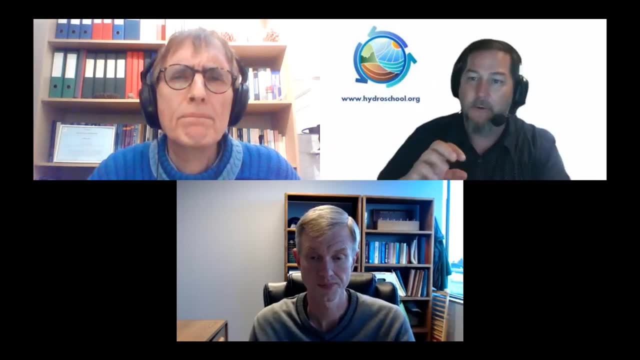 with those tubes going straight down. all we got to do to look at surface water where velocity heads up. what does become important is we just curve that tube at the bottom, point it like a pitot tube into the flow and then we raise up by that velocity head. 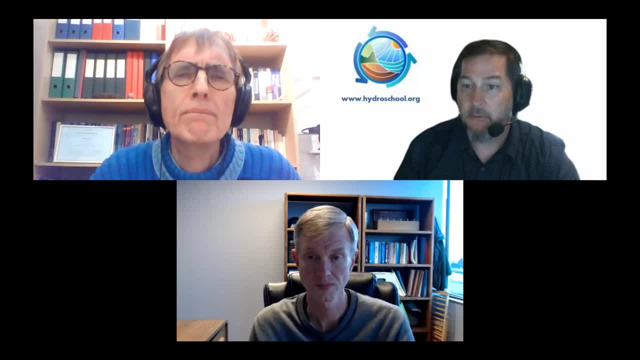 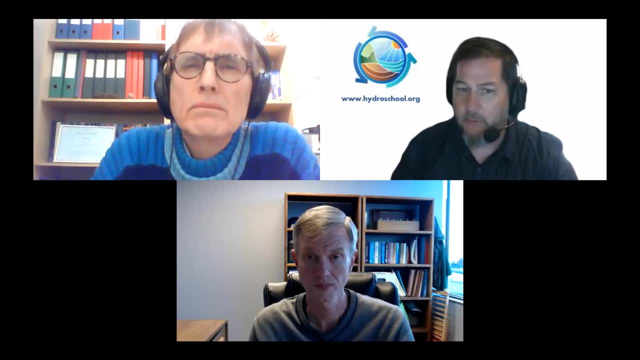 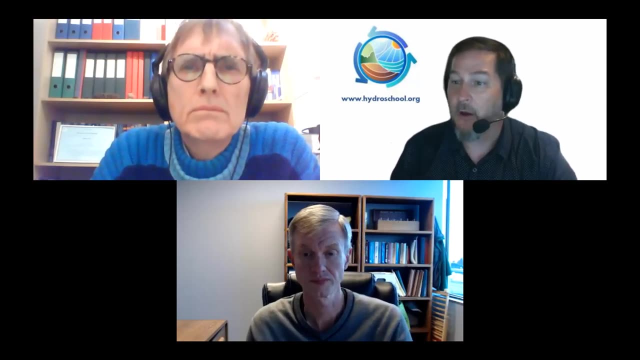 So there are a lot of these concepts that we're seeing here that do go back and forth between surface water and groundwater and the principles that we cover. So maybe first Guy and then follow up with a final answer from Dr Hendrix here The questions that came in regarding confined aquifers: 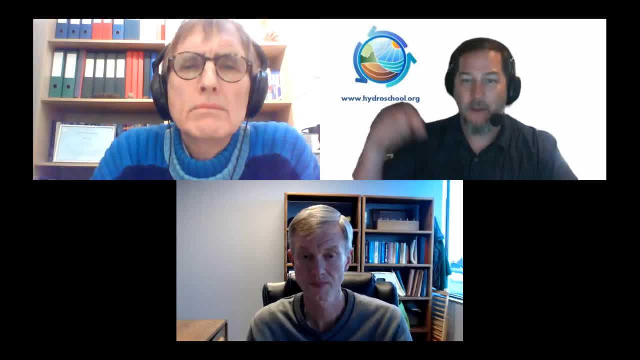 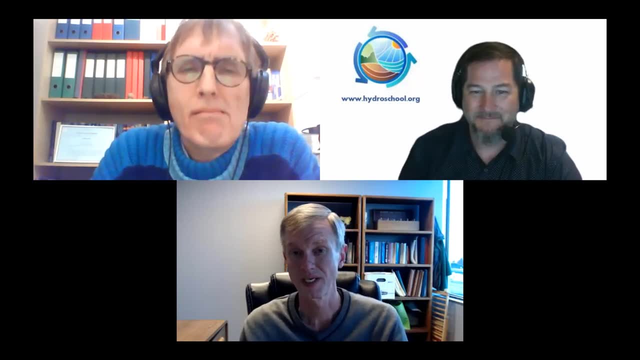 what would the signs be? How would you be able to tell when you start punching holes in the ground? how can you tell if it was a confined aquifer? So, Guy first and then over to Dr Hendrix. Yeah, And I was answering just in a typical sense. 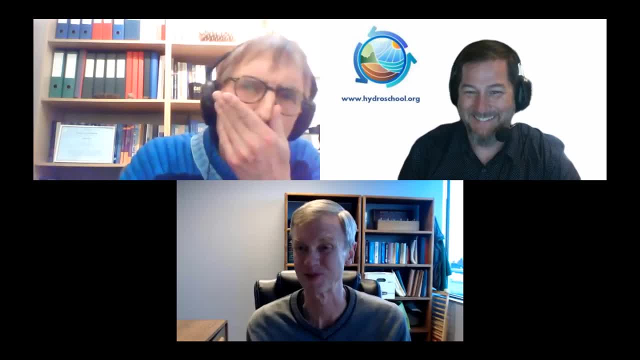 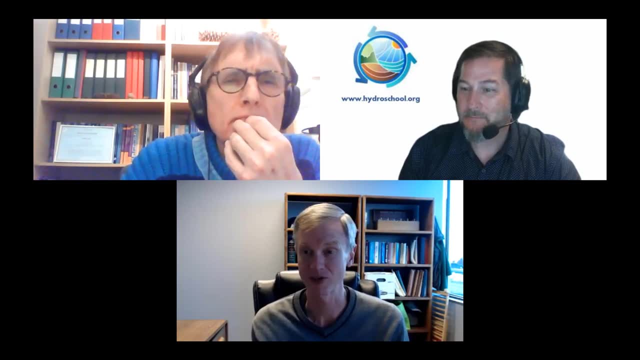 And some people chimed in with some very specific examples. But typically you install a well or a piezometer, you measure that hydraulic head that was discussed in this seminar and you compare it to the top of the aquifer and you see if it's under confining conditions or not. I mean, that's in the most general typical sense. Now there's obviously some exceptions, but that is typically. you find that the pressure at depth is higher than it is more shallow, So it's under confining conditions. Or if the well flows, then you have artesian conditions. 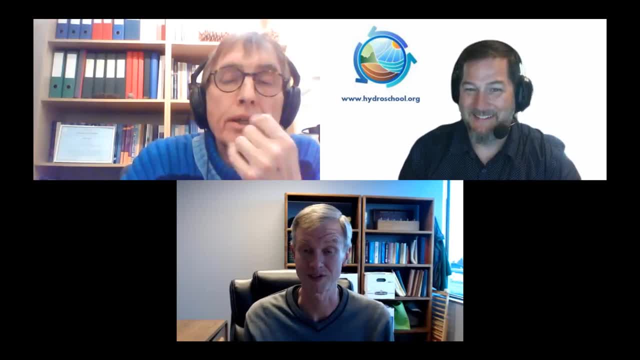 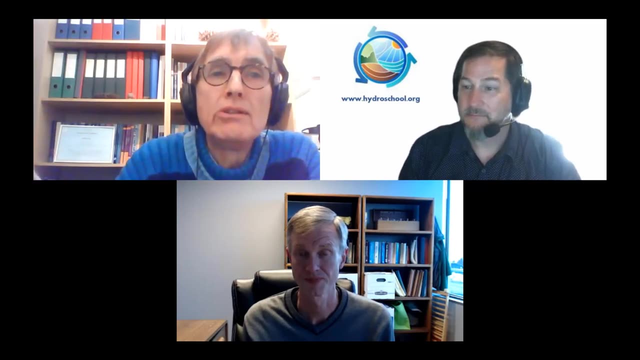 and you definitely know it's confined. So that's another example. Yeah, And also the relation you find between the piezometers is a linear relation, that's in confined groundwater. Yeah, It's actually the most easy, easiest case to model confined groundwater flow. 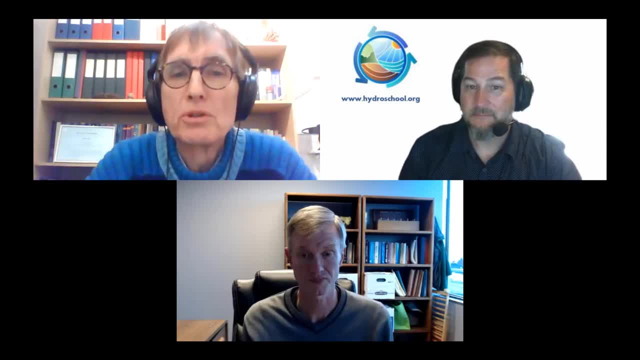 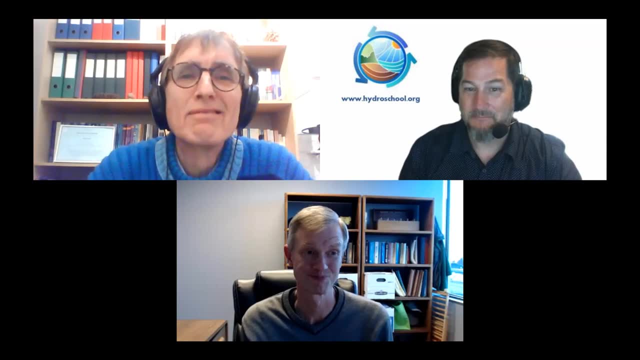 In the course. we'll start off with confined groundwater. Yeah, So groundwater models converge a lot if you're under confined conditions in aquifer, Yeah Yeah, All right. Well, we'll have some practical examples for you in the course. 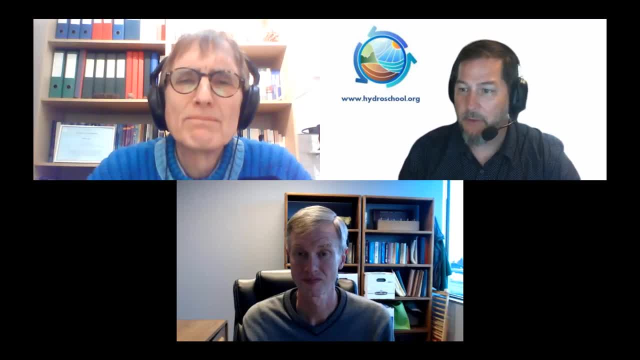 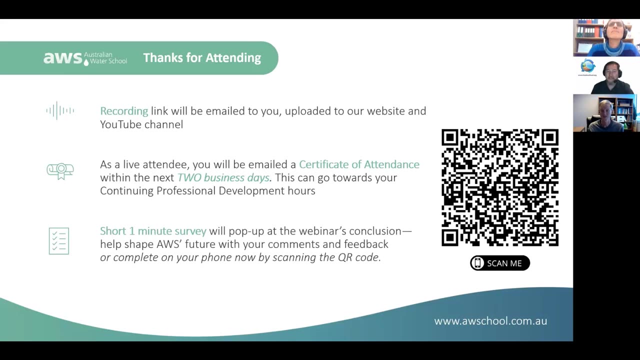 We'll also follow up with additional webinars that cover groundwater and contaminant transport and some things like that, And we will respond to your further questions and feedback as well. So thanks to everyone who joined us. Thanks especially to Dr Hendricks for coming on at the late wee hours of the night. 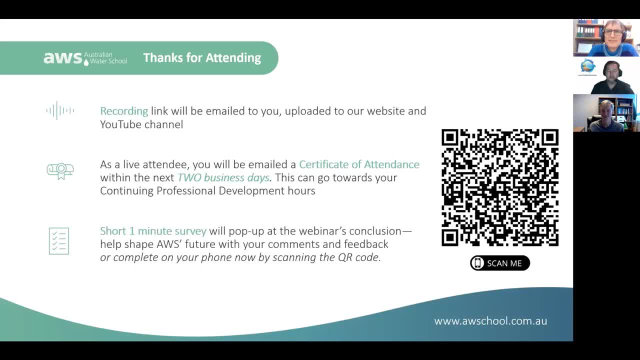 in the Netherlands. We try to get an international focus for these and perspective for these courses and for all of our webinars And for something like this. it's obvious from a lecture like today why you can receive certificates of attendance. So if you need registration support, 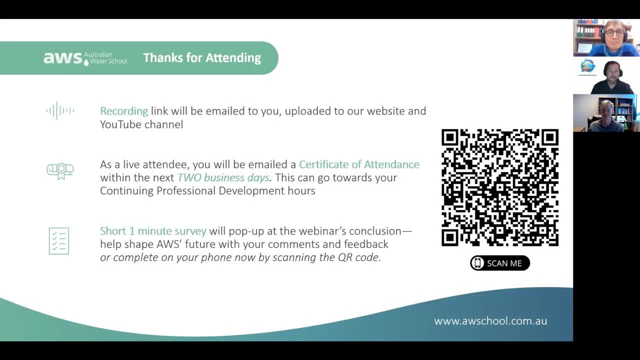 and things like that for your certifications and your licensing. you can earn those by attending these webinars and these courses, And in some cases this is like going back to school. For me, that's a bit of a refresher. My last groundwater course was probably 25 years ago. 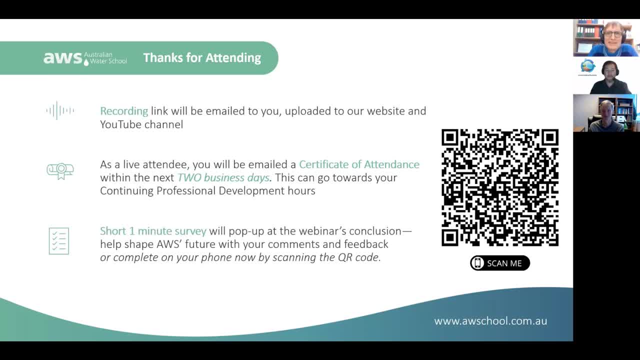 but I deal with groundwater on a daily basis. Sometimes it's inflow, sometimes it's outflow from my surface water models, but we've all got to interact. We want to promote the groundwater, surface water interaction realm, whether our models are good at doing that or not. 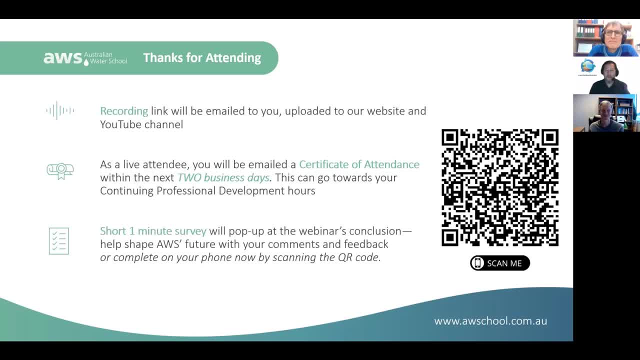 We want to make sure that we're accounting for all of the principles that we need to know about when we start opening models and throwing numbers into these variables. We want to make sure we've taken away the mystery of the black box. So thanks so much for your attendance. 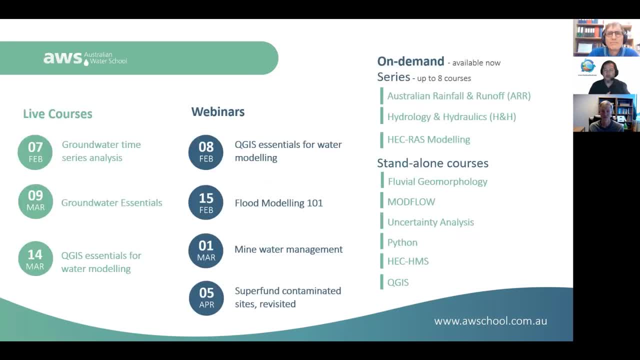 You'll see a couple of links here. come up for some future courses and webinars. Promote these in your social networks, if you can. We like to bring you the content, the best content that we can and the most relevant content to your work. 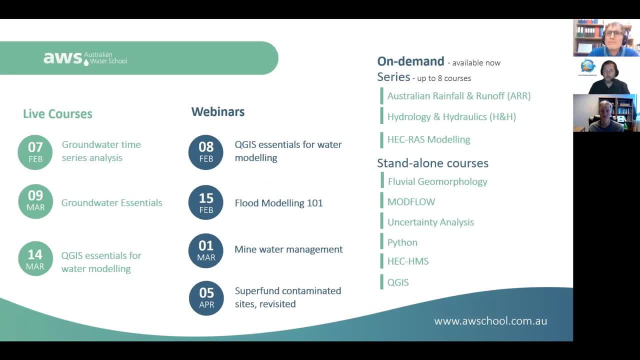 So thanks so much for everybody for attending. Thanks. Maybe I'll let you guys just give your final goodbyes and closing remarks here, But thanks These lecturers and presenters and panelists come on As volunteers. we're interested in furthering the industry here. 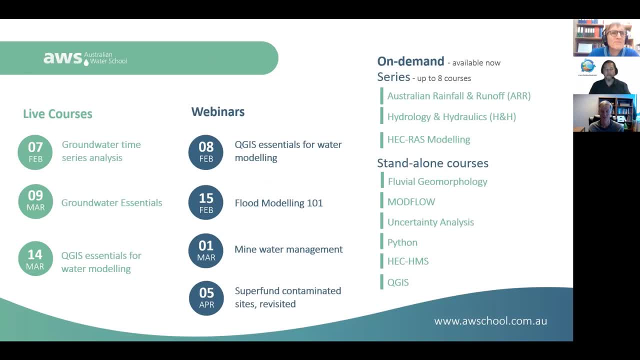 but our feedback from you is the pay that we get for our time spent here with you And we do value that And it is something that we like to promote, going forward, this contact with the industry. So, Guy, closing remarks, and then over to Martin to close it off for us. 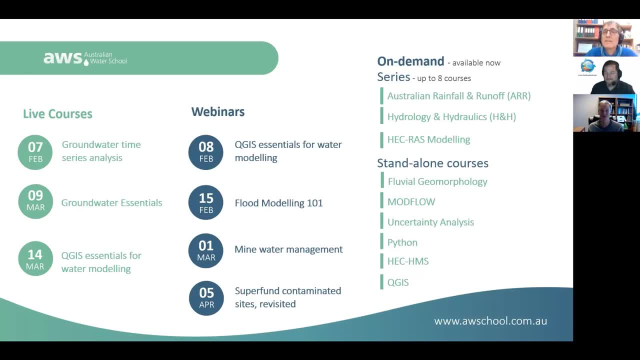 Yeah, Just as a groundwater modeler, I'd like to say: when your model is not doing what you think it's doing, you always go back to first principles like this in the conceptual model and see if something is not correct. So it's an important foundation to establish.